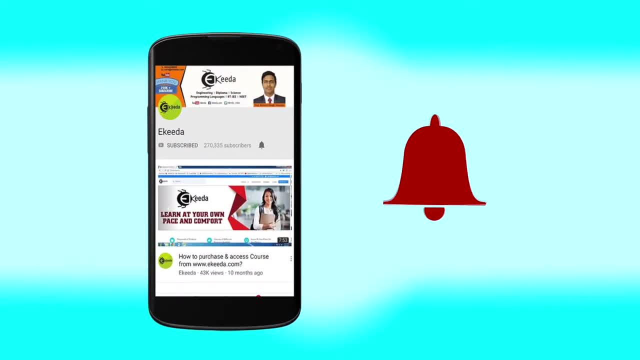 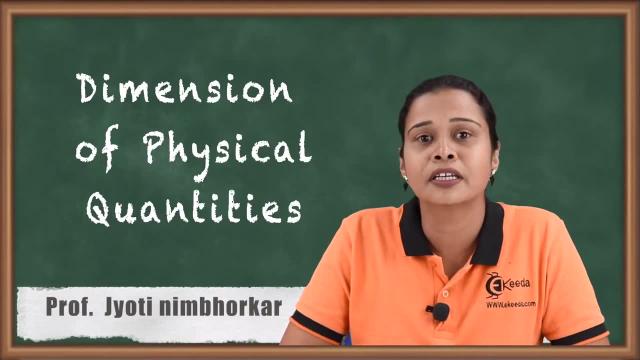 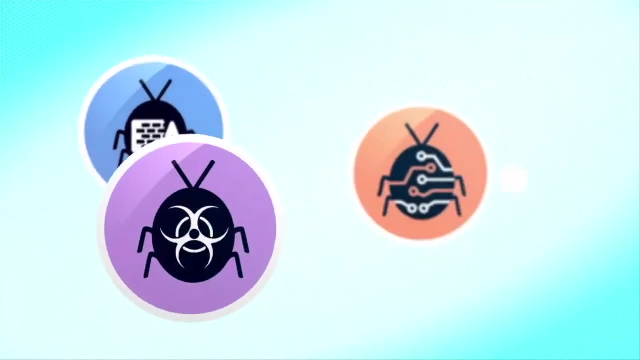 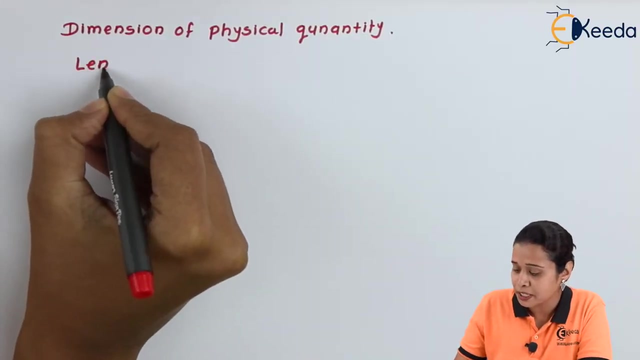 Click the bell icon to get latest videos from eKIDA. Hello friends, today we will see dimensions of physical quantity In mechanics generally, basic three quantities are length, mass and time. So here length can be expressed in terms of capital L. 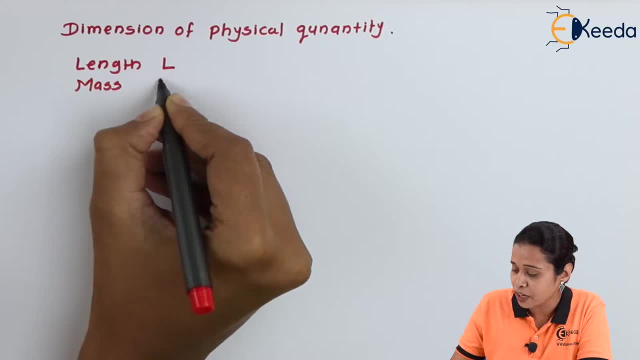 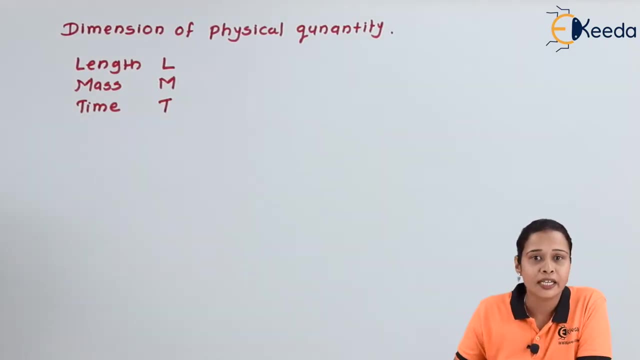 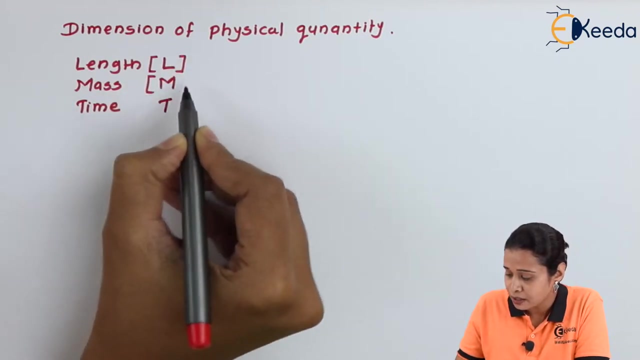 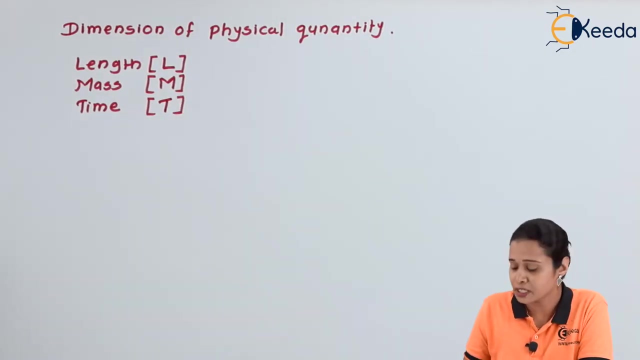 Mass is expressed in terms of capital M and time is expressed in terms of capital T, And we always write dimension in square bracket, So the dimension of L will be in the square bracket like this. So first thing we will find out here: dimensions of physical quantity. 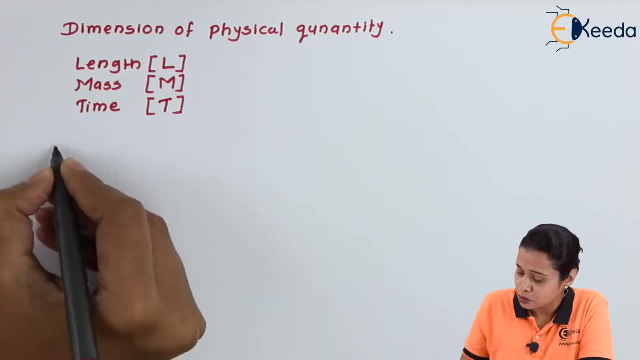 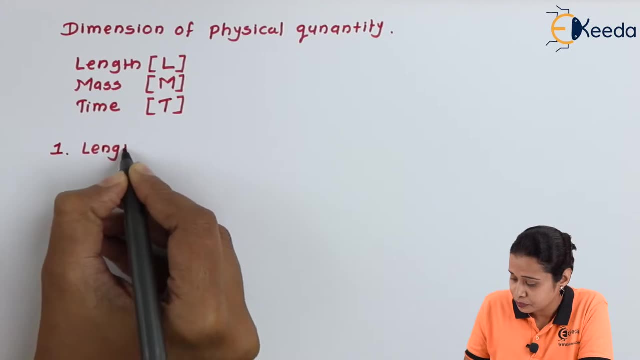 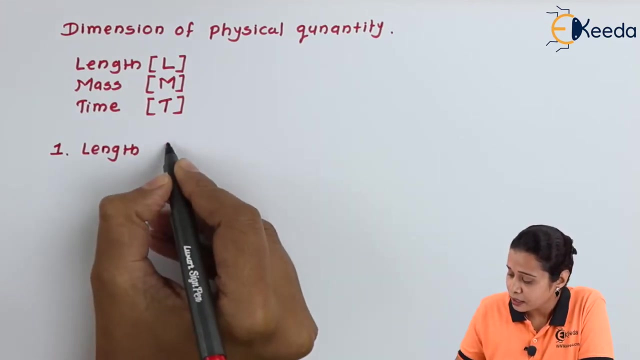 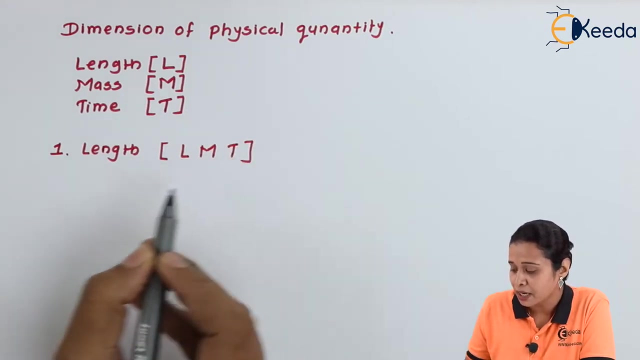 and first quantity we will consider that is a length. So let us start from that. What are the dimensions of length? So we will write here. So first physical quantity: we will take length. to find the dimensions So length, here we will take L, M, T, that is length, mass and time In case of length. 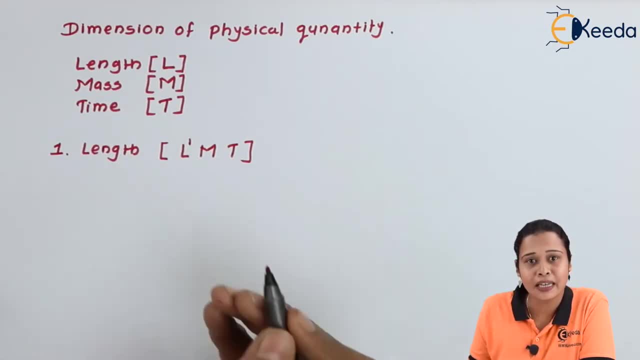 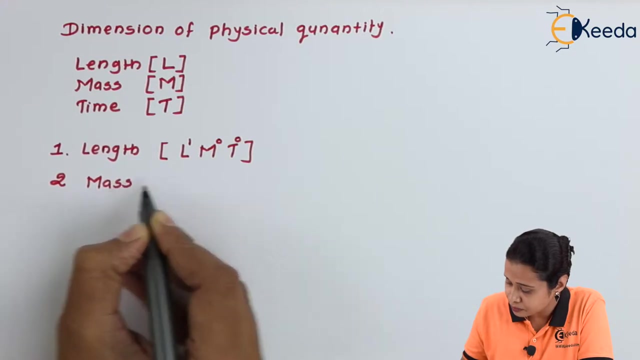 here we will write down power 1, because in length length is present, but mass and time is absent, So we will write down power 0.. Next physical quantity we will take, that is a mass. Again the same way we will write, that is M, L, M and T. Here length is absent, So it is 0. 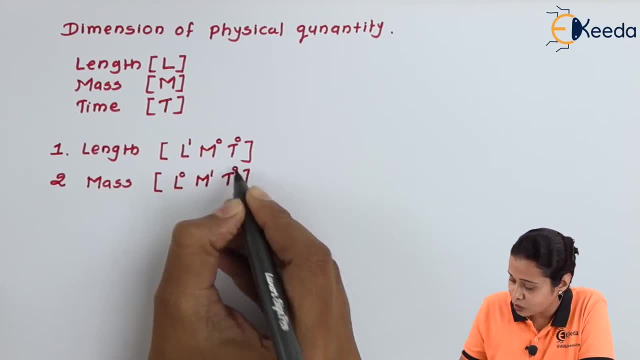 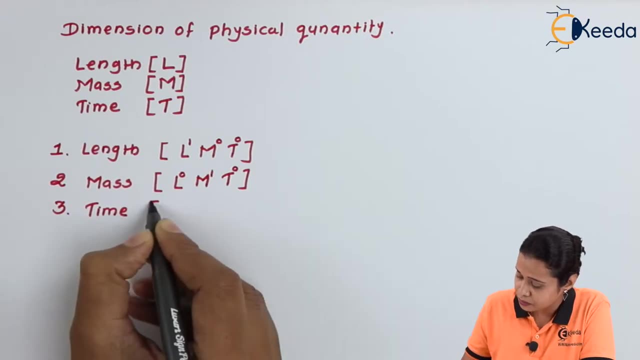 Mass is there, So it is 1, and time is not there, So it is 0.. The third physical quantity we will take, that is a time In time. length is absent, So it will be power 0.. Mass is also absent, So it is 0, and then time. 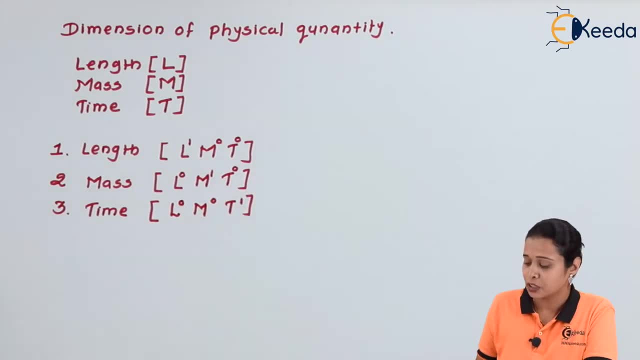 is present, So we will take here power 1.. So these are the three basic physical quantities. The next physical quantity we will take, that is area. We know area is equal to length into breadth. Length and breadth, both we can express in terms of L. So here we have L into L, which is equal to. 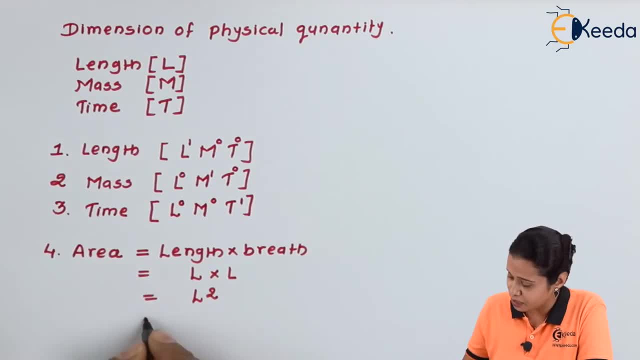 L square. Hence the dimension of area can be written as L raise to power 2.. M, that is mass, is absent and time is also absent And if you want to write down the unit, then from this we can write unit of area that is meter square. 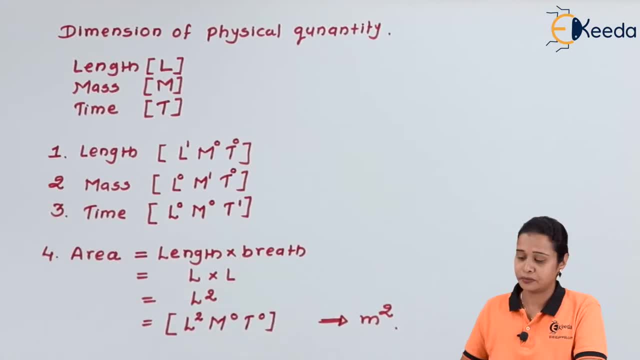 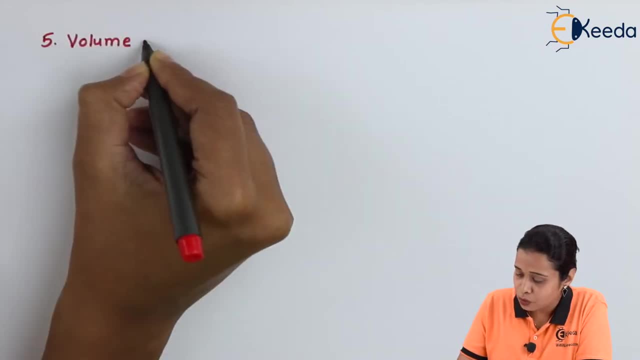 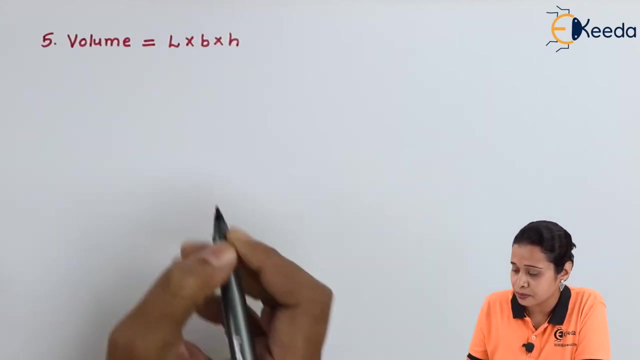 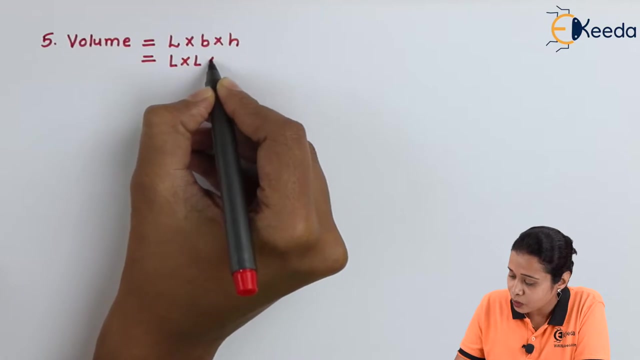 square. next, physical quantity we will take for the dimension that is a volume. we know volume. the formula of volume is length into breadth, into height. so here all these three terms we can express in terms of length. so here we can write down length into length, into length. 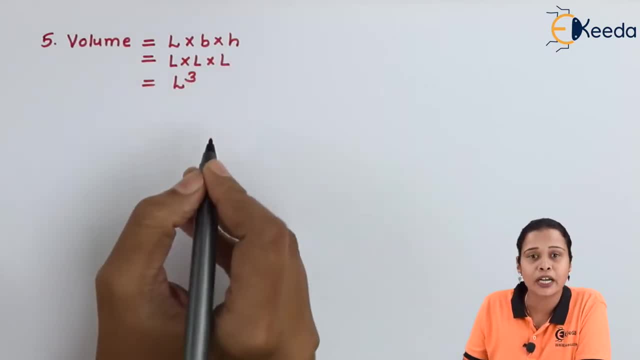 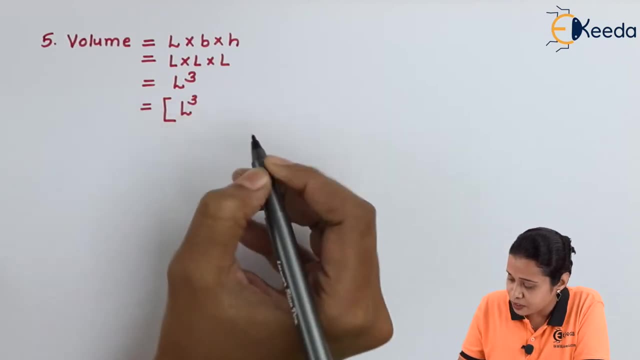 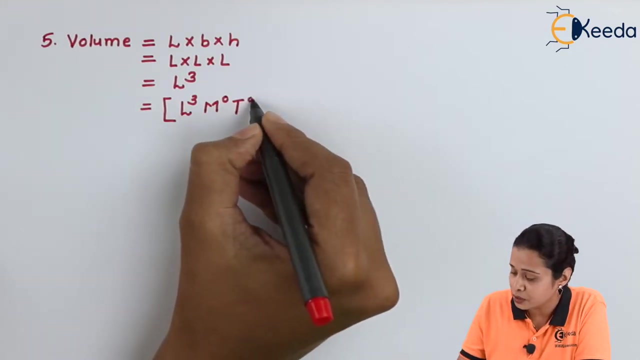 that is equal to l cube. now, if you want to write down the dimension of volume, we will write down in a square bracket. so l is to the power 3. mass term is absent here, so we will write down 0. time is also absent, so we will write down 0. and if you want to write down the unit of this, 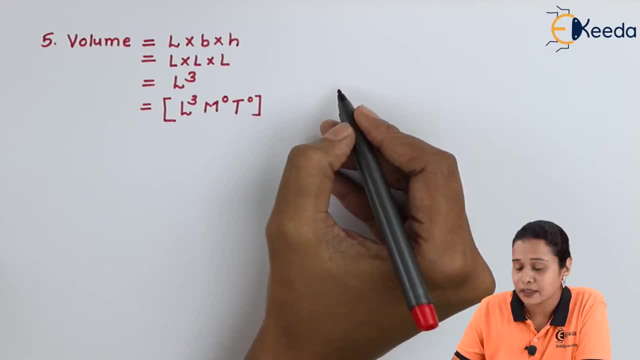 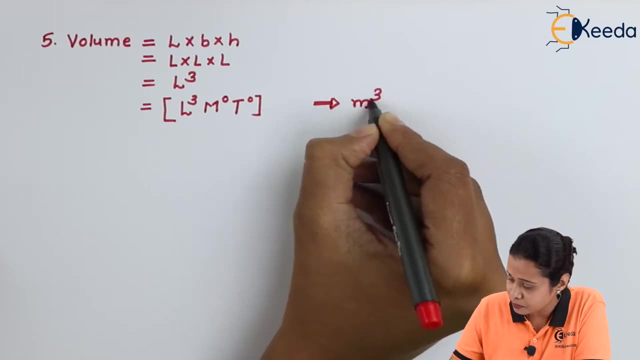 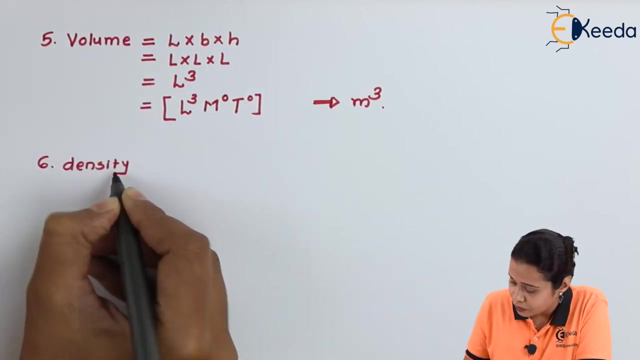 so l cube l is nothing but length, and that length is expressed in terms of meter. so the unit for this is: is meter cube. next, physical quantity: we will take that is a density. we know what is the formula of density: density is nothing but mass per unit volume. 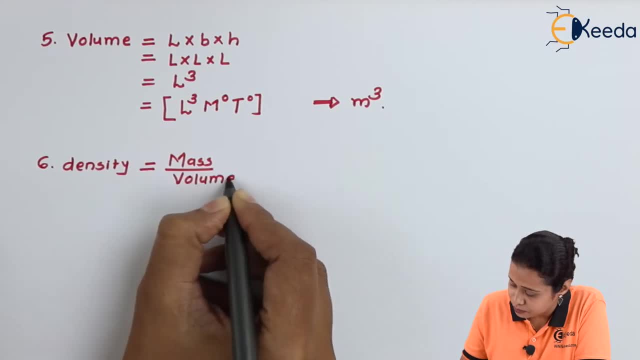 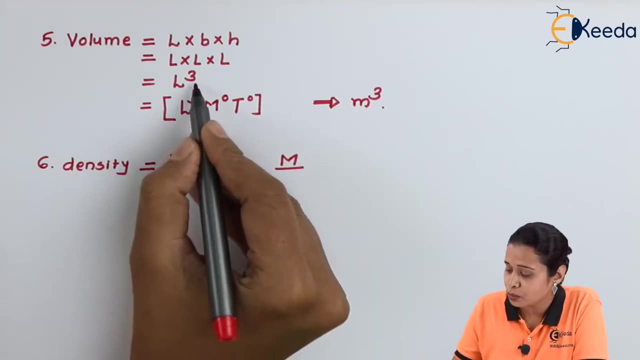 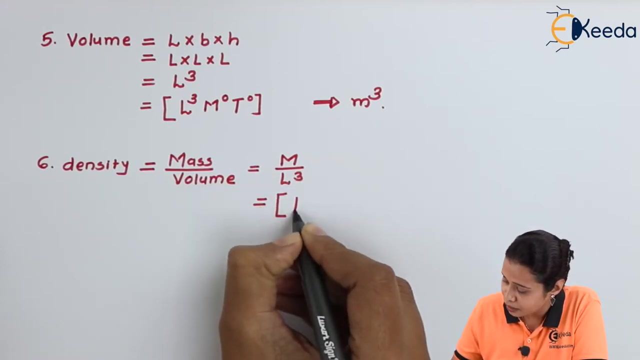 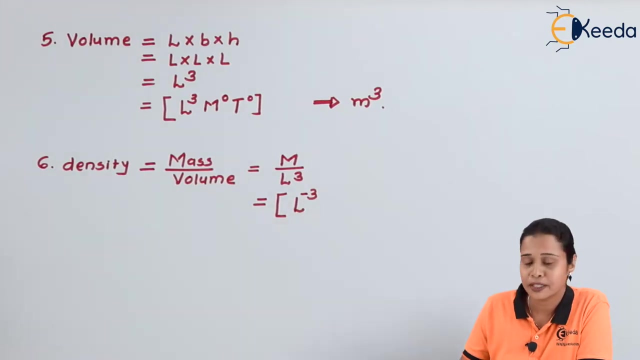 so we will write down here mass, that is m, and volume- we can express volume in terms of l cube. hence, dimension of density is l, but now l is in the denominator, so we will write down here minus 3, that is to the power, minus 3. 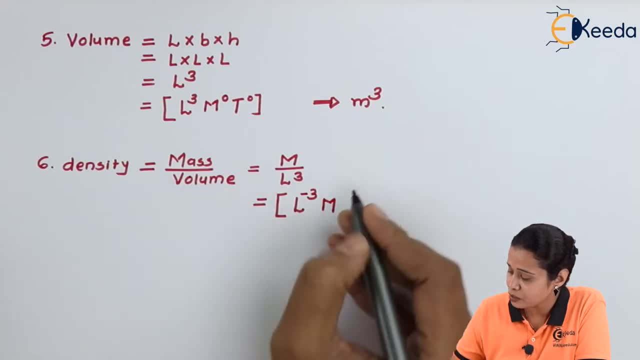 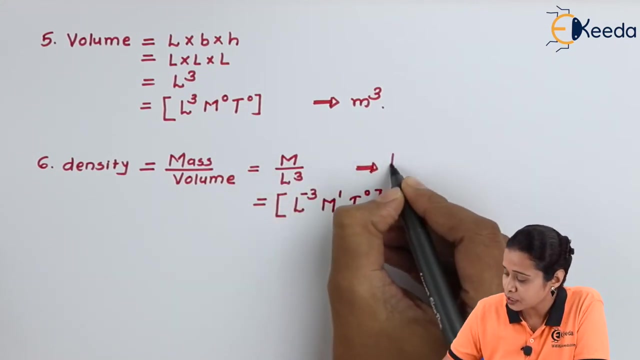 the mass quantity is present there, so power of m is 1, but t is absent, time is absent, so we will write down 0. if you want to write down the unit of density from this, we can write down. this is a mass. we know what is the unit of mass, that is kilogram. 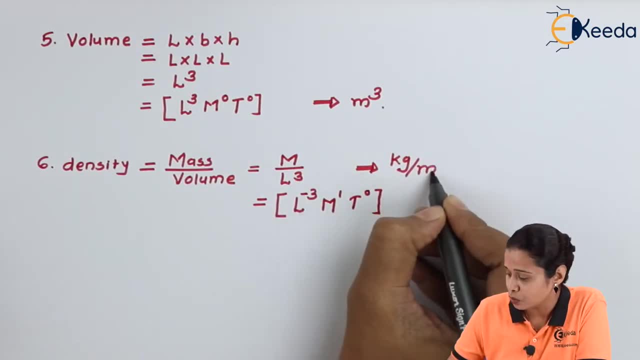 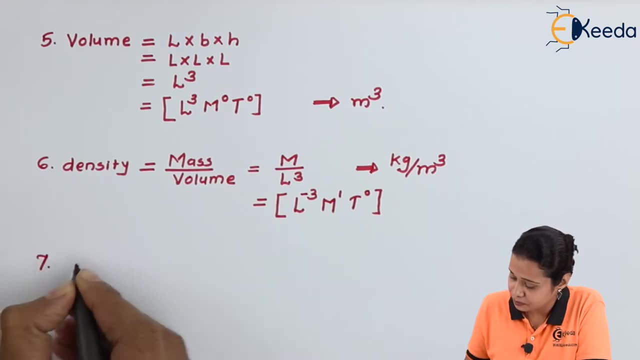 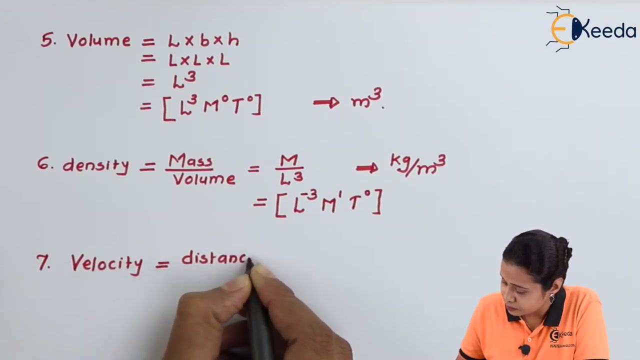 and this is length cube. length cube is nothing but meter cube, so this will be the unit of the density. next physical quantity we will take, that is a velocity. we know velocity is distance per unit time. so here we will express distance in terms of meters. so here we have a quantity that is a length. 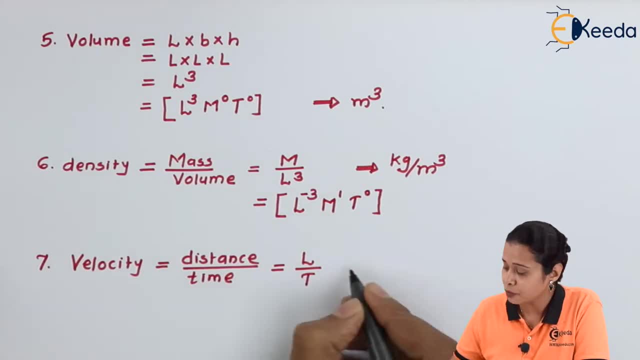 and we will write it down. here we have a length. and time means here we have a t. so if you want to write down the dimensions, here dimensions are l1, t is in the denominator, so here mass is absent firstly, and t is in the denominator, so it is minus one. 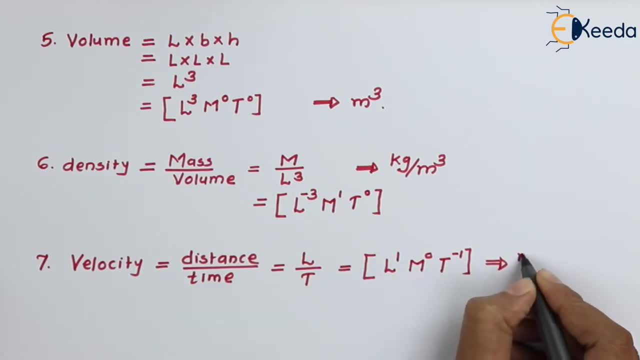 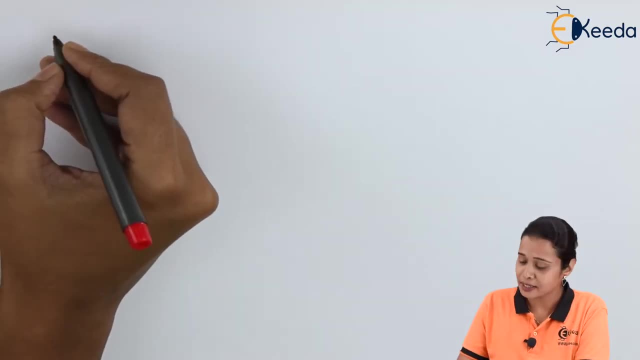 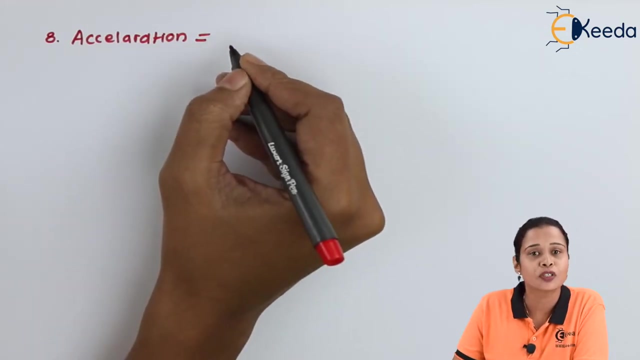 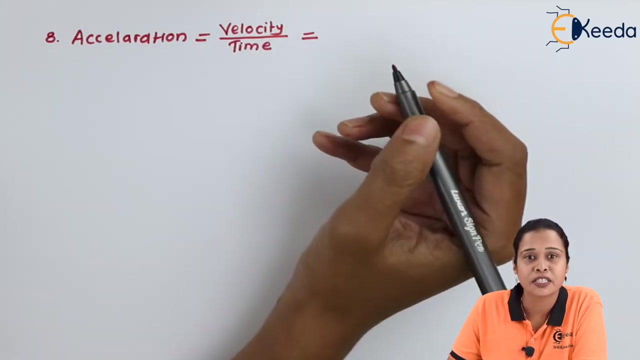 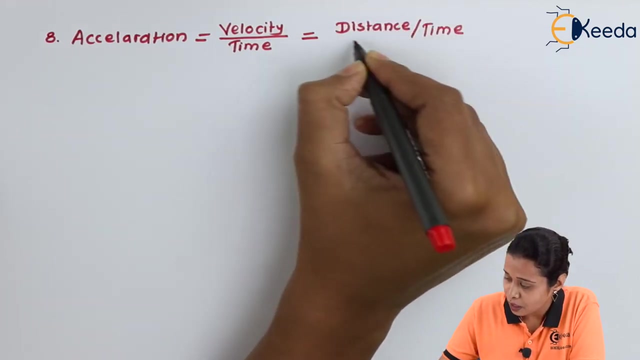 and if you want to write down unit, the unit for this it's length. l is length, means meter and per second. Next physical quantity we will take, that is acceleration. We know acceleration is velocity per unit time We can express. velocity is distance per unit time upon time. 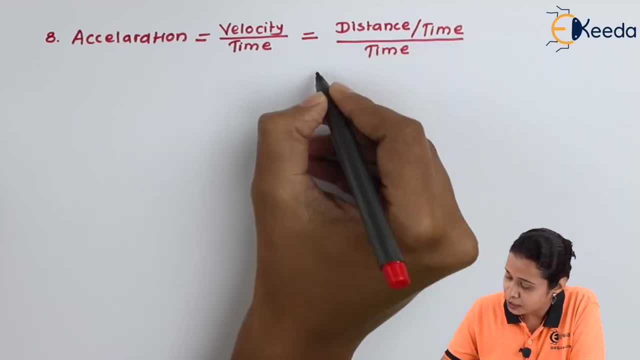 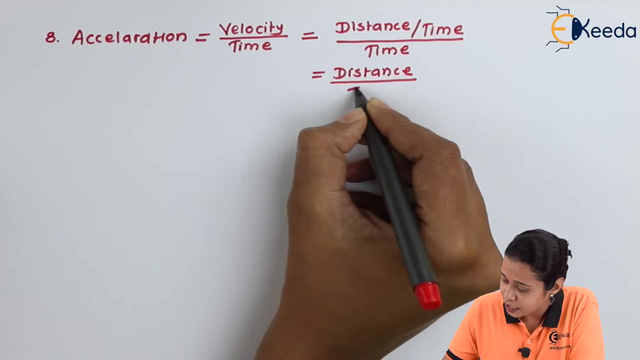 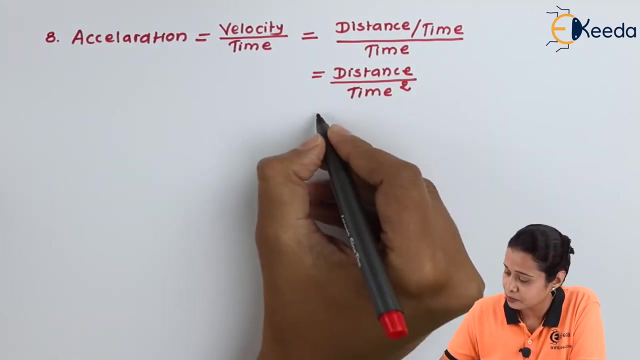 So here we have a formula that is distance per unit time square. Now we can express distance in terms of L and time in terms of t. So here we have a t square. So if you want to write down dimensions, we will write down in this way. Firstly, we will take a square bracket. 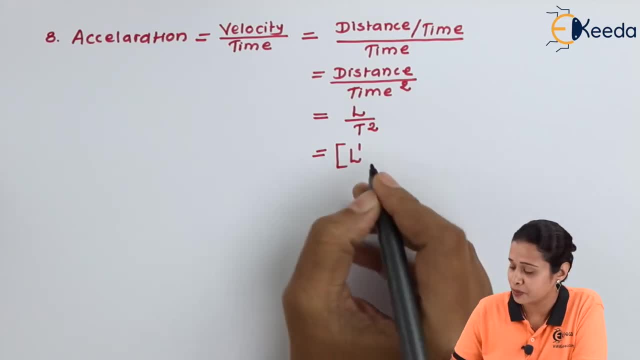 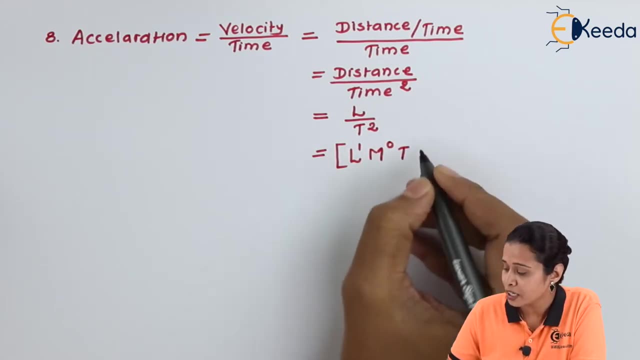 and we will write down a square bracket. So here we have a square bracket and we will write down a square bracket. Then L1, power of L, will be 1.. Mass factor is absent here, So here we will write down m0. and here t is in the denominator, So we will write down: 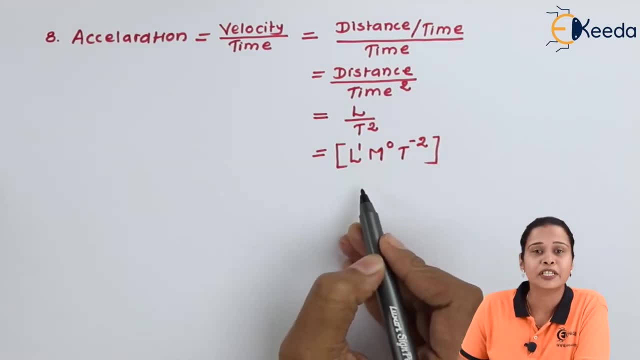 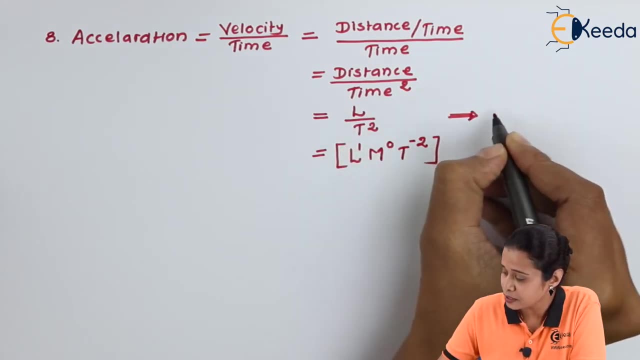 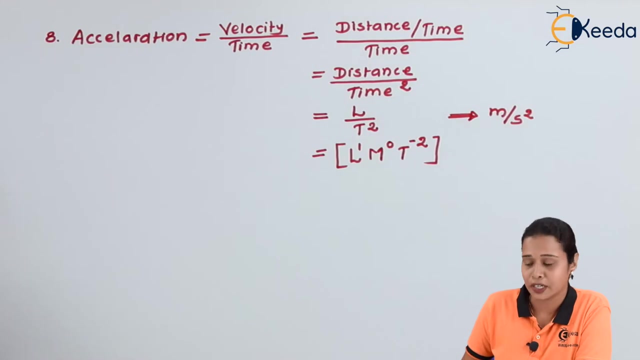 here minus 2.. This is the dimension of acceleration. If you want to write down unit, then here length can be expressed in terms of meters and time in terms of second, and here time square. So this is the unit of acceleration and this one is a dimension of acceleration. Next, physical: 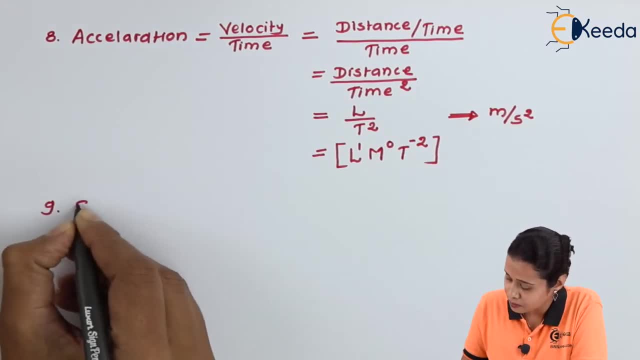 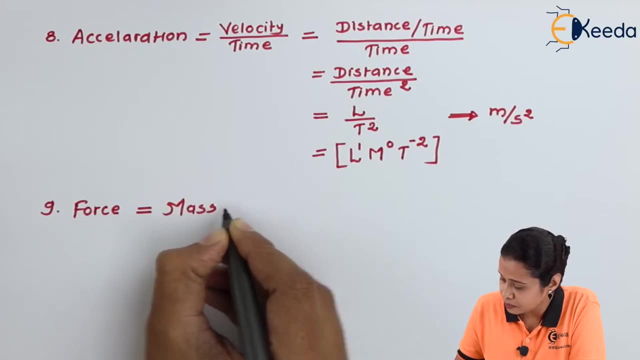 quantity. we will take, that is a force- We know force is equal to mass- into acceleration. So here acceleration again can be expressed in terms of velocity per unit time, And again velocity can be expressed in terms of distance per unit time. So final equation: 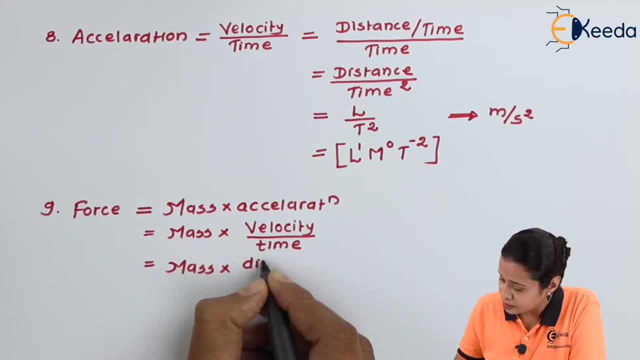 will be mass into distance upon time square. Hence here we have a factor that is m. Distance is nothing but length here, and time is t, that is a t square. So the dimension for this physical quantity will be L1.. Mass is present here, So we will. 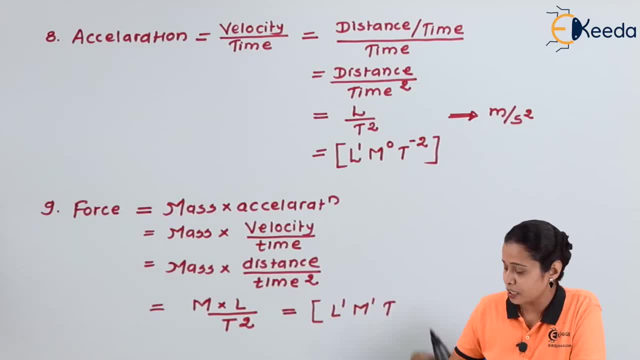 write down m1 also, and t is in the denominator, So we will write down minus 2.. This is the dimension of force. Now, if you want to find out the unit of force, we will find out from this equation. We know mass can be expressed. the unit of mass, that is a kg. kilograms Distance is in. 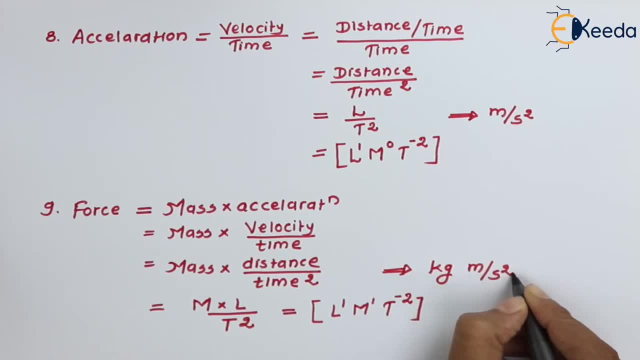 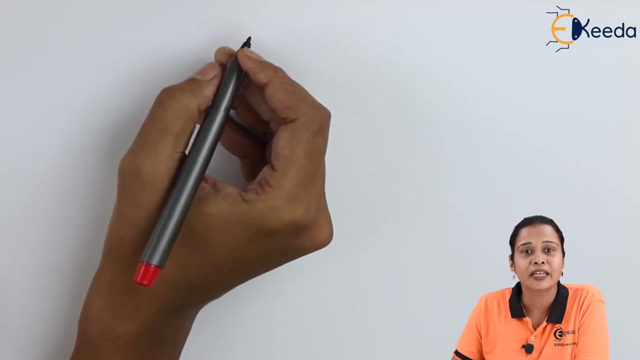 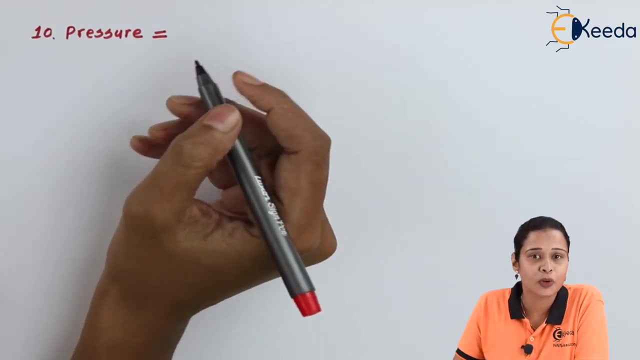 meter, And then time is in the second. So here we have a second square. So this is the unit that is, kg meter per second square, is a unit of force and the dimension is in square bracket L1, m1, t minus 2.. Next physical quantity we will take, that is a pressure. We know pressure is force upon area. 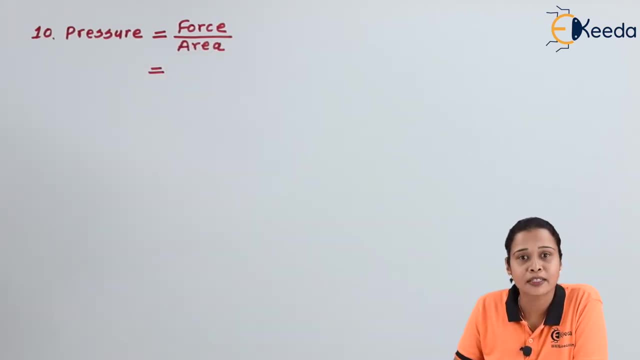 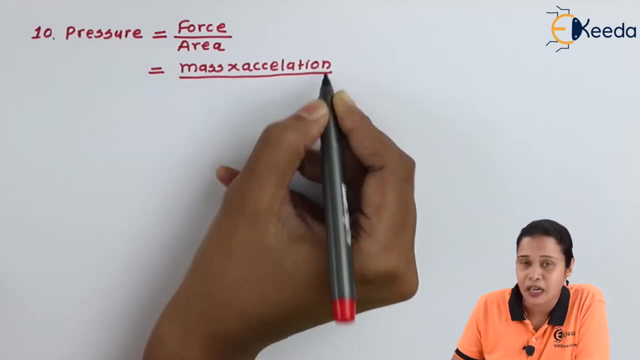 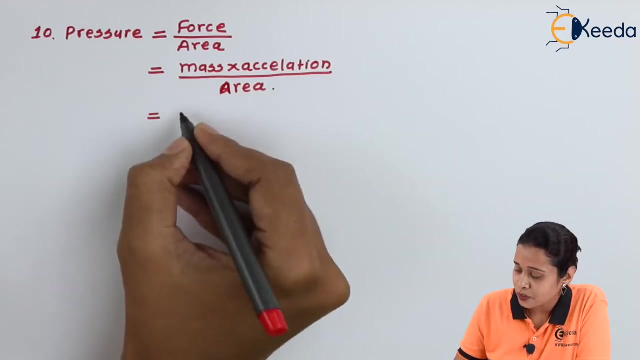 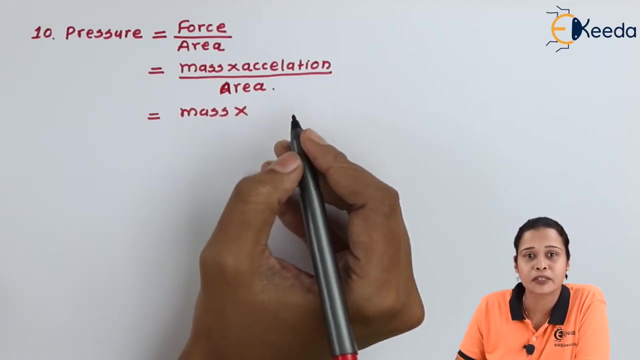 Now, force can be expressed in terms of mass into acceleration. So we will write down mass into acceleration and here upon area. So we will write down here mass acceleration. again, we will express in terms of velocity per unit time, And here upon area. 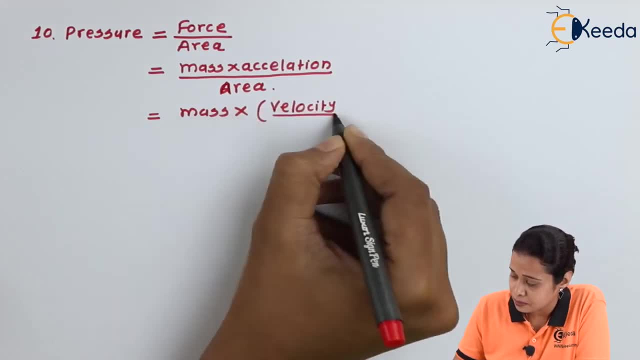 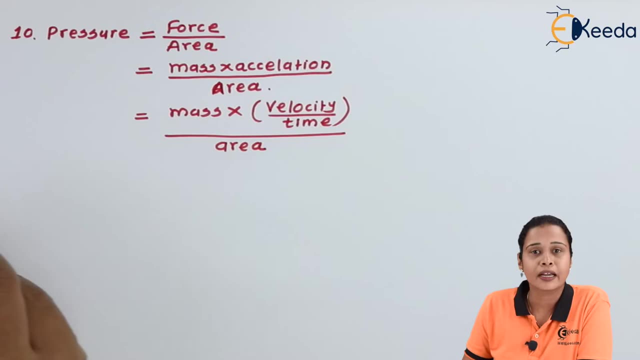 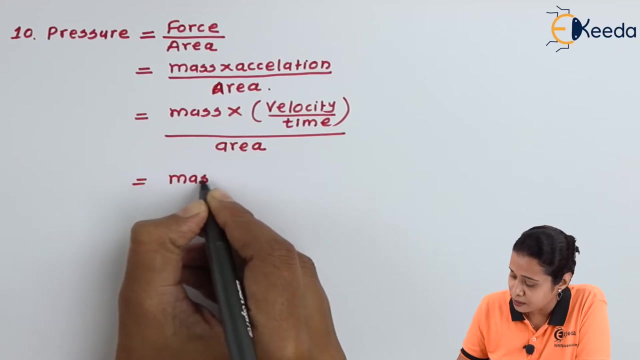 So we will write down here mass acceleration again we will express in terms of velocity per unit time. And then we have a area, Again velocity can be expressed in terms of distance per unit time. So finally we will write down this equation: mass into velocity, that is, distance per unit time. 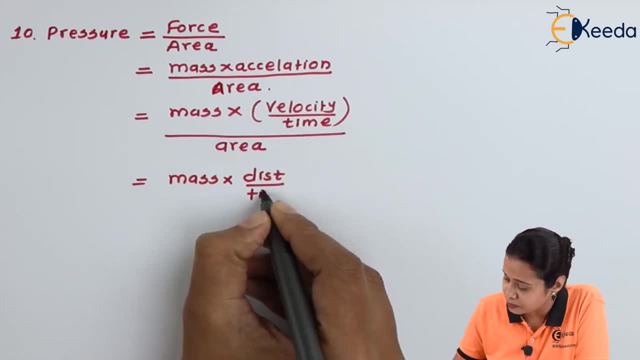 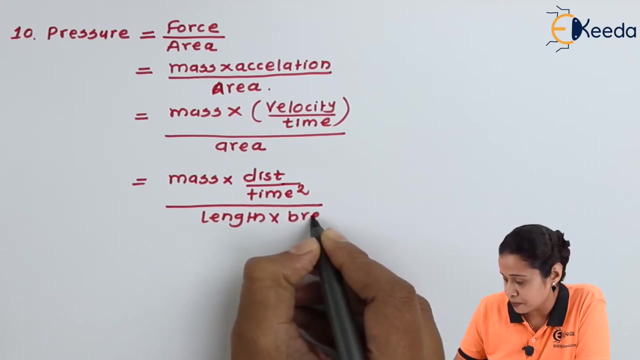 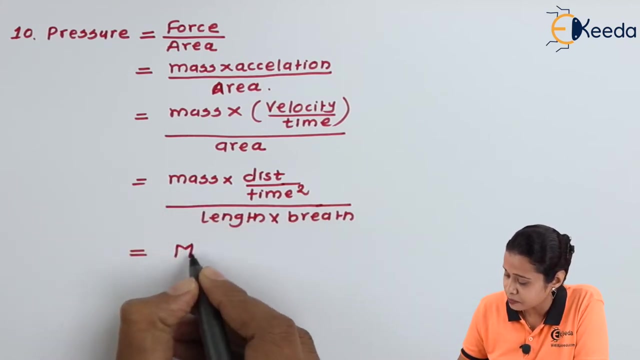 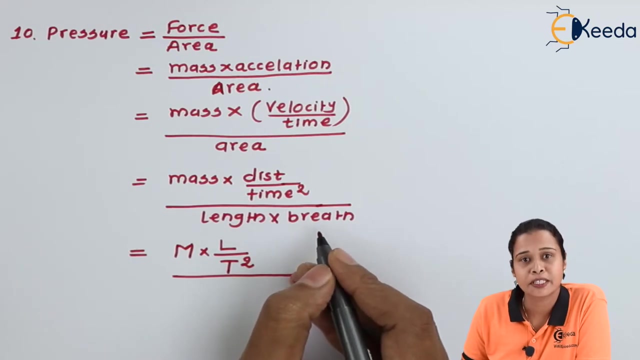 means here distance upon time. square and area is nothing but length into breadth means. here we will write down length into breadth. So finally, mass, that is m, distance, we will express in l, and time, we will express in t, that is t square. here Length and breadth, both can be expressed. 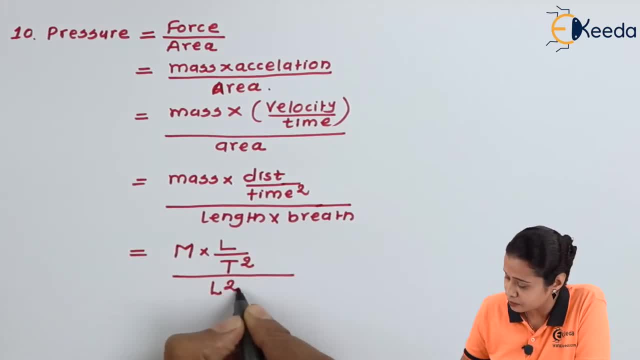 in terms of L. So we will write down here L square. So finally we will have here this: L will get cancelled. So here we have M upon L into T square. So the dimension of pressure is L is in the denominator. So we will write down: L minus 1, power of M will be 1 here. 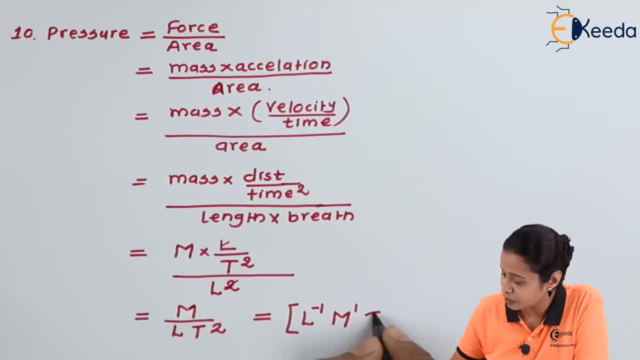 and T again is in the denominator. So we will write down T raise to minus 2.. So this is the dimension of pressure. If we want to find out the unit, we will come to this equation. For the unit we will write down this is kg. Mass will express in terms of: 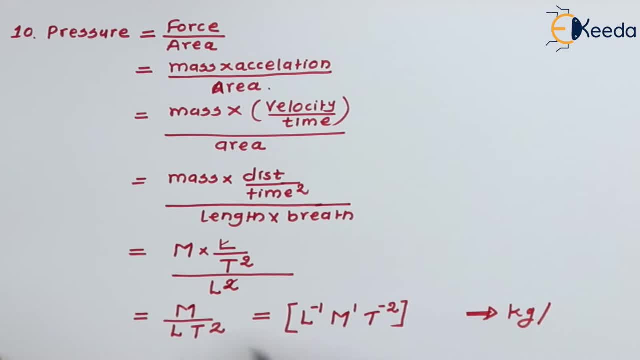 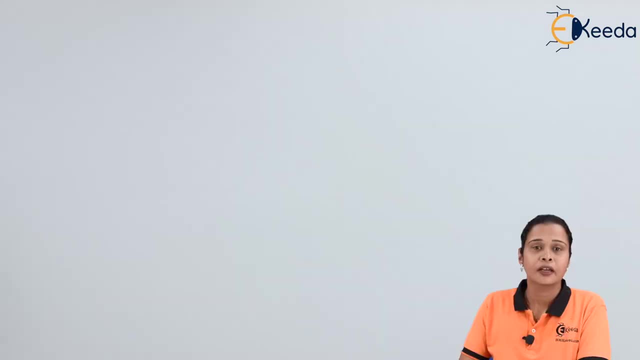 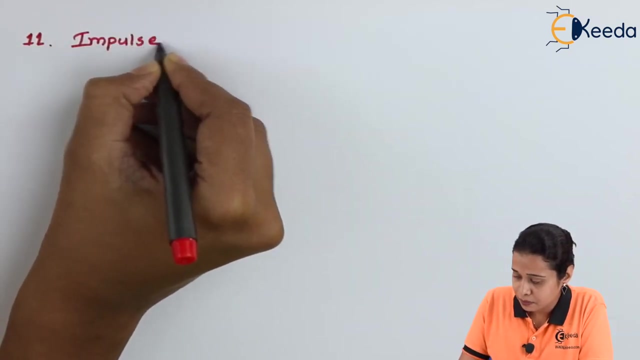 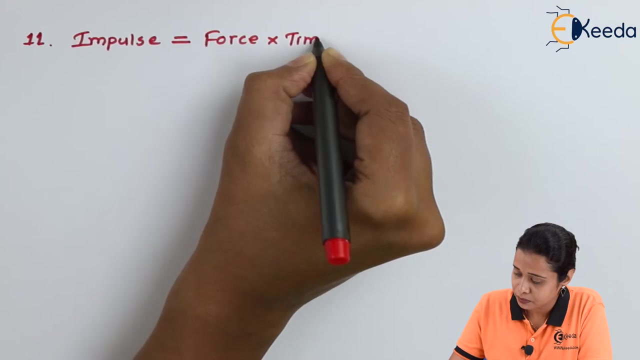 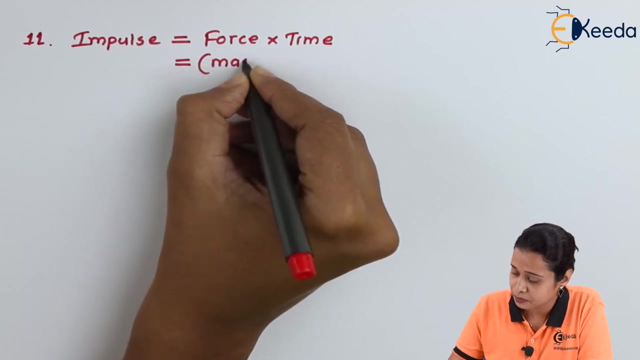 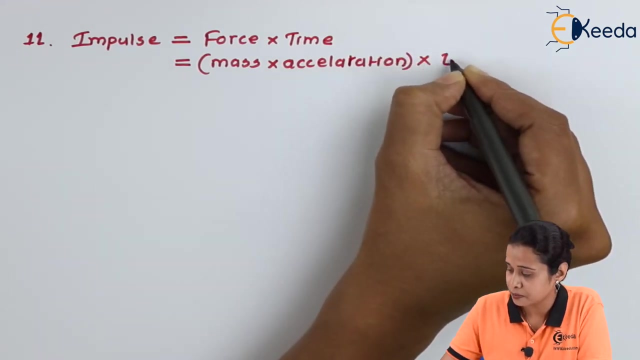 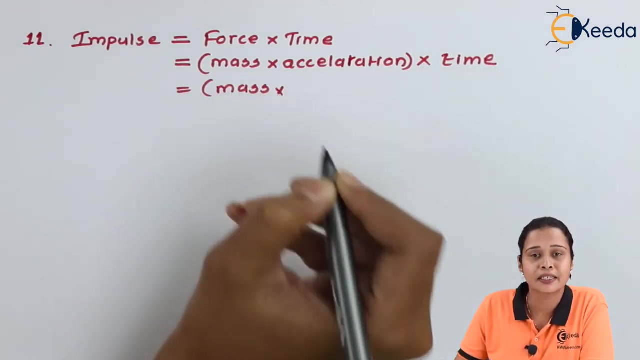 kg per unit length, that is meter and second square. So this is the unit of pressure. Next physical quantity is impulse. We know impulse is force. into time, Force can be expressed in terms of mass, into acceleration, into time. Again here, acceleration can be expressed in terms of velocity per unit time. 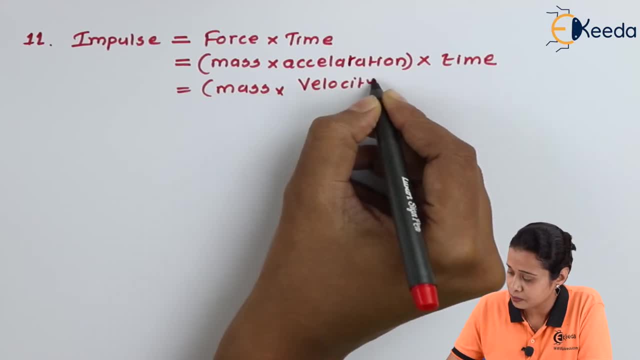 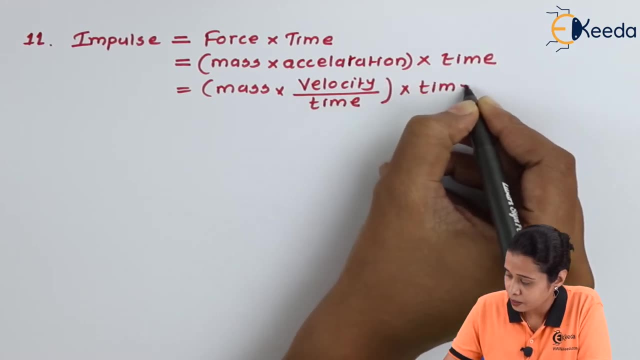 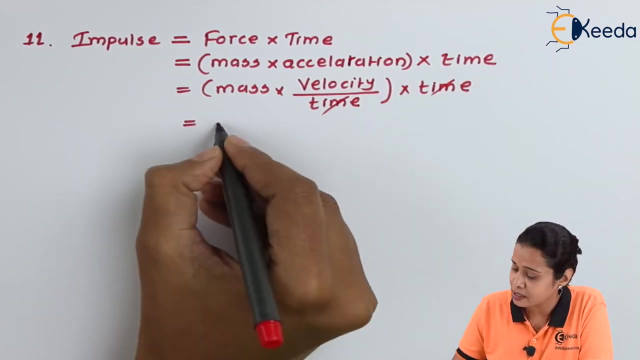 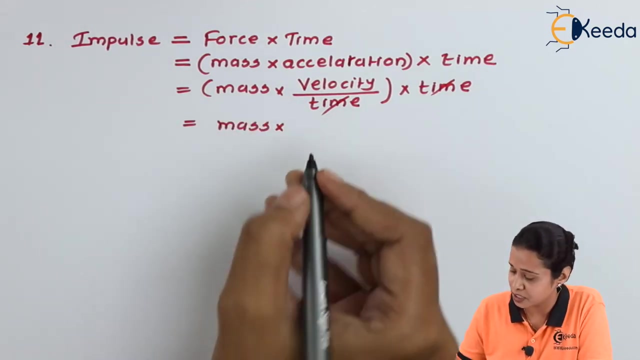 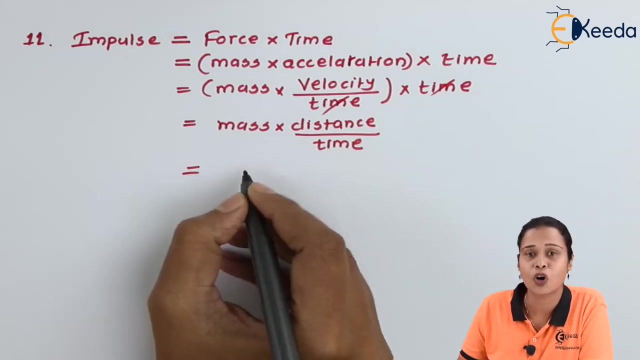 into time. In this equation, time factor is getting cancelled. Now here this equation can be written as mass into velocity. Velocity is again displacement or distance per unit time. Hence here we have a quantity, mass, that can be expressed in terms of M. Then we have 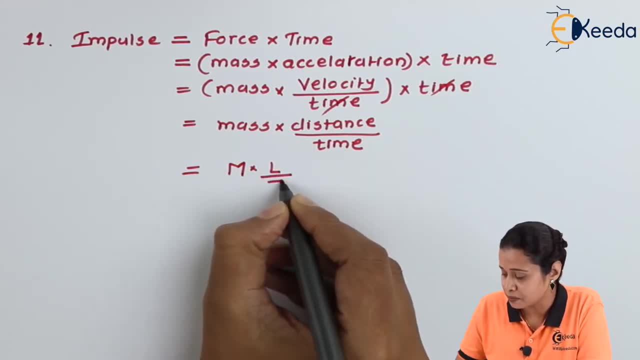 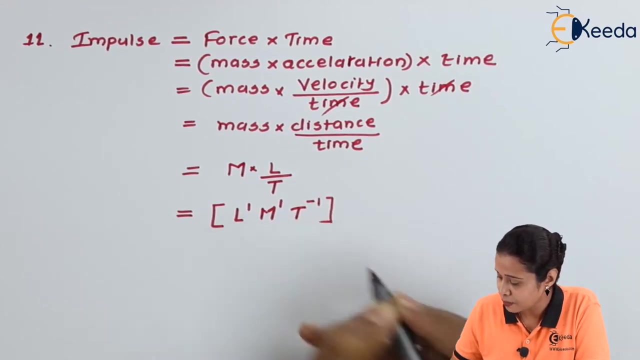 a distance, that is L, and then time. Hence the dimension of impulse can be written as L1- M1.. T is in the denominator, So we will write down T minus 1.. If we want to find out unit of impulse, we can find out from the above equation For 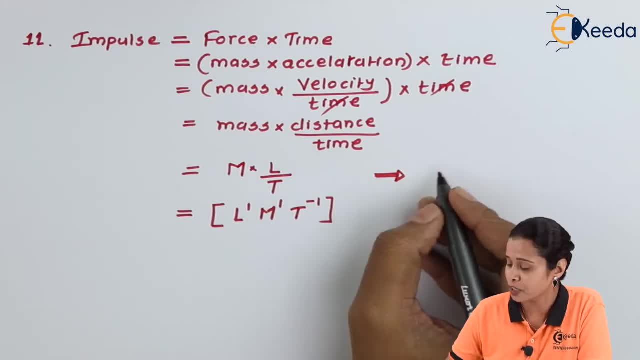 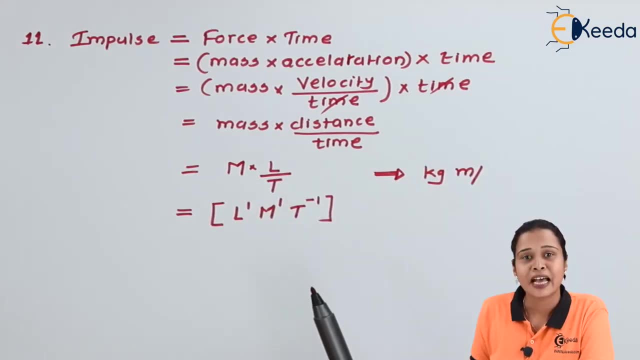 unit M, that is, a mass, can be expressed in terms of kilograms. Length can be expressed in terms of meter. Hence the dimensions of impulse is L1, M1 and T minus 1.. If you want to find out the units of impulse, we can find out from the above equation, So we can write. 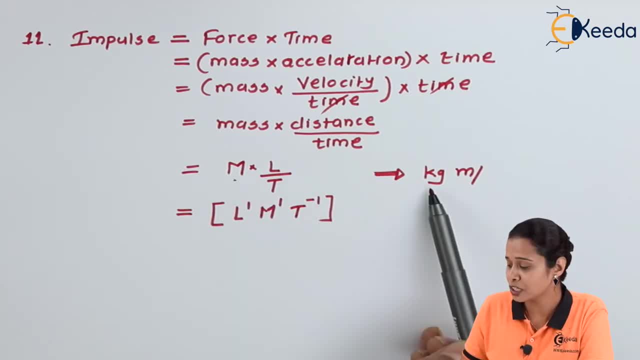 down M. Here M can be expressed in terms of kg. So here we have a kg. Length is in meter and then time is in the second. So unit for impulse is kg, meter per second. Next physical quantity is a work. We know work is force into displacement. Force can 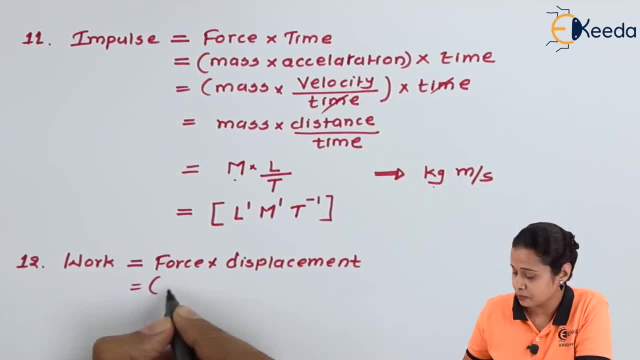 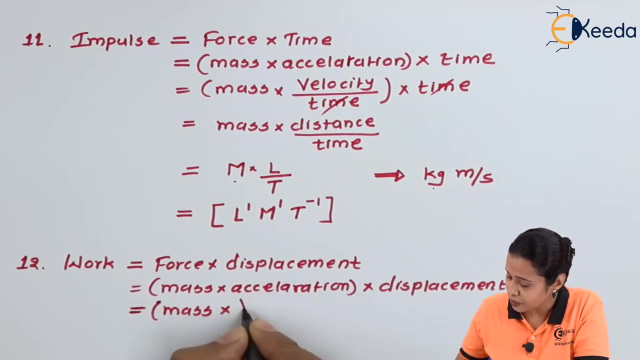 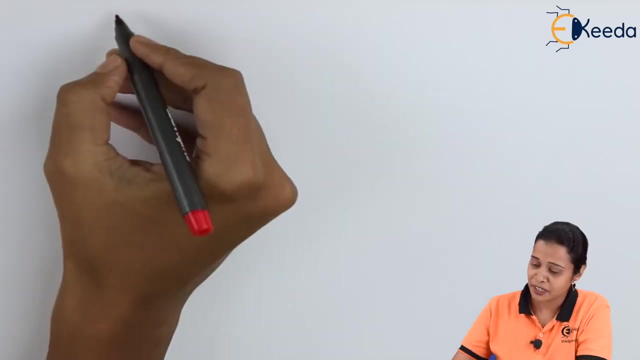 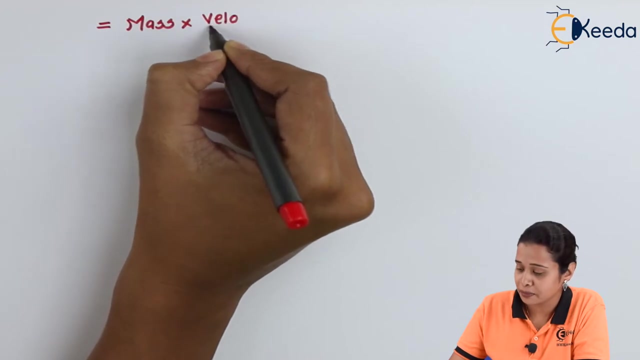 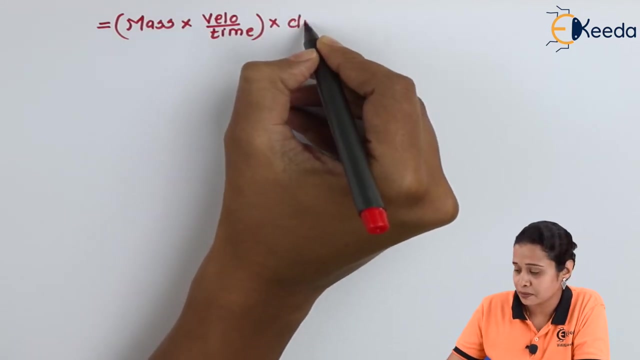 be expressed is equal to mass into acceleration. Here we know, acceleration can be expressed in terms of velocity per unit time. So here we will write down mass. Acceleration is velocity per unit time into displacement. So here we will write mass into velocity per unit time into displacement. We know very. 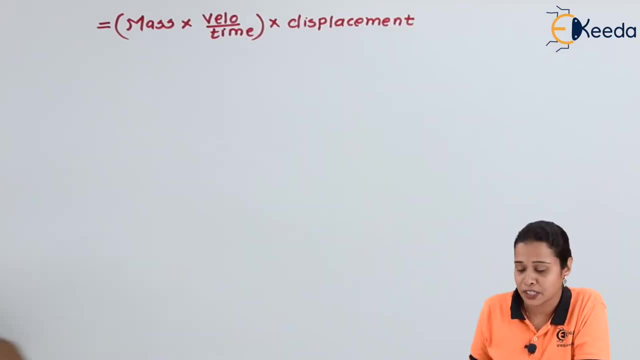 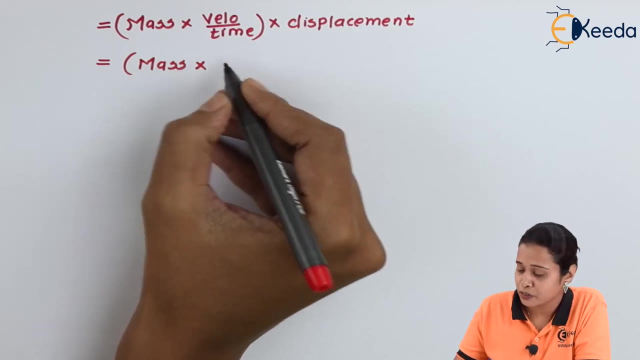 well. So we know velocity also can be expressed in terms of distance per unit time. So directly we will write down here mass Eat Water into distance per unit time. So we will write down here distance per unit time and this time 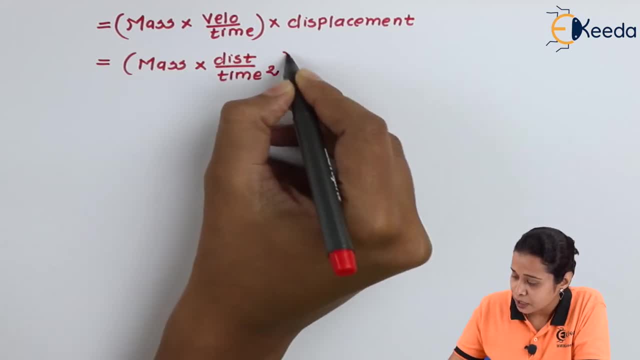 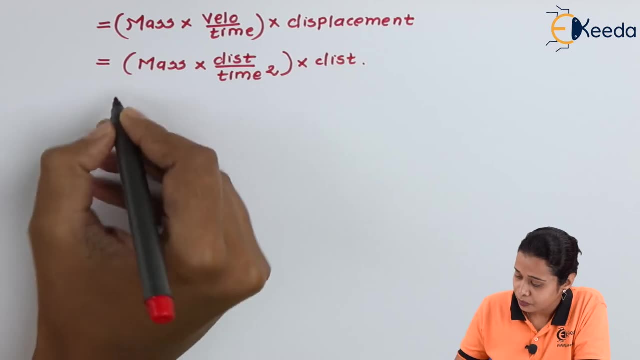 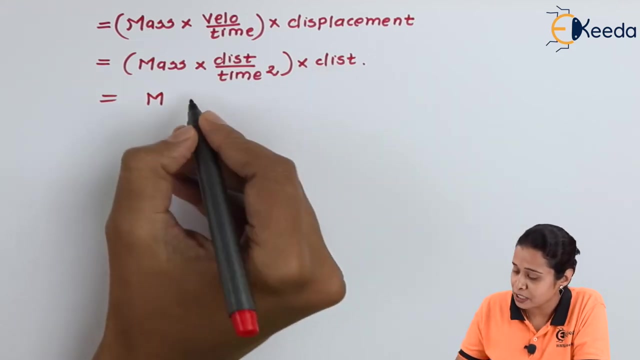 is also there. So time square into displacement. Displacement is nothing but distance. So we will write down here distance. Now here we have a terms, that is m for mass. Then here we have a two time distance means what L square upon t square. 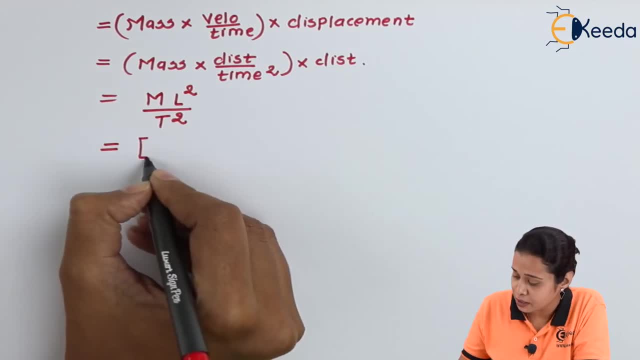 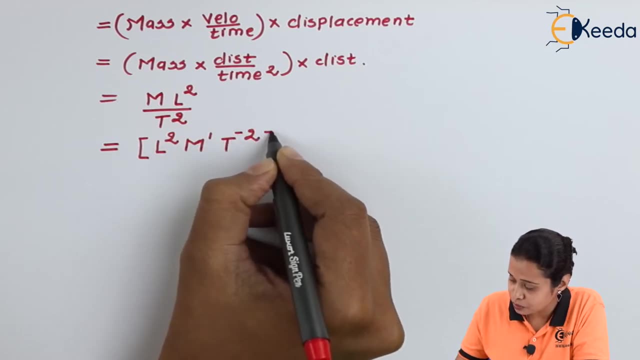 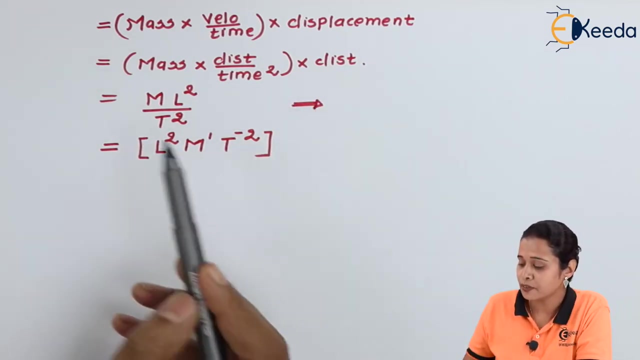 Hence the dimension for this quantity will be L square m1, t minus 2.. And if you want to find out units for this, we will write down unit from this formula. Here we have a m. m is nothing but mass. 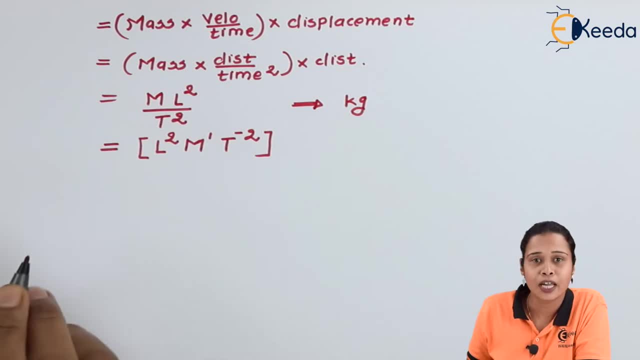 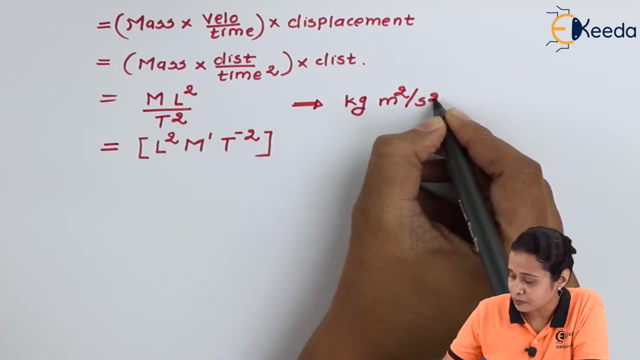 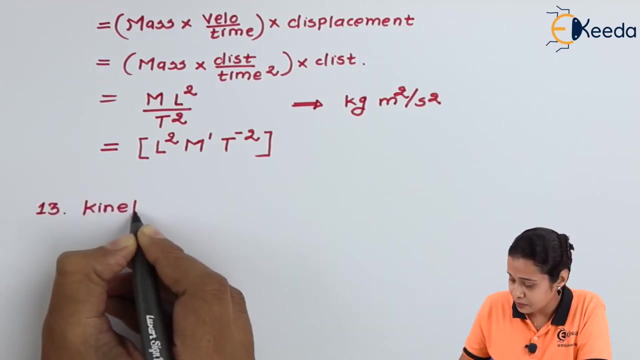 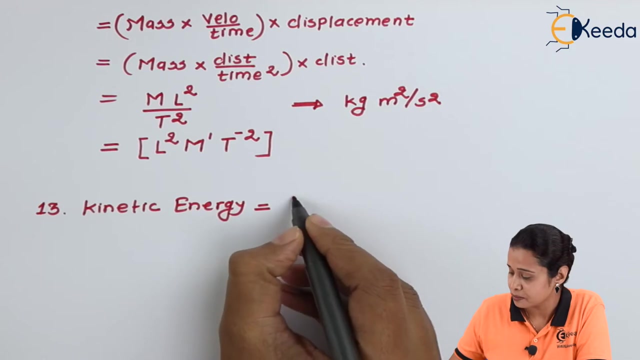 So unit for mass is kg, Unit for length is meter, So here length square, So meter square upon t square means second square. Next physical quantity will be kinetic energy. We know kinetic energy is equal to half mv square, that is half mass into velocity square. 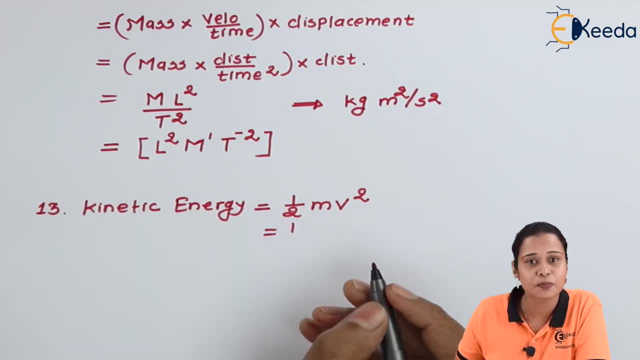 So we will write down here distance per unit time. So we will write down here distance per. We can express velocity in terms of distance per unit time. So here we will directly write half m. distance per unit time. square, whole square. Now we will write down here half m. 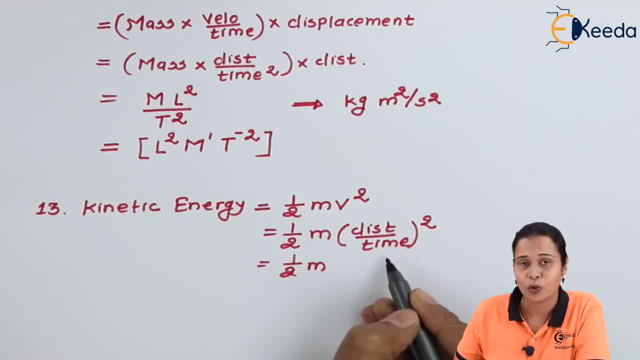 Now, distance is nothing but length. So length, square upon time, square. So we will write down here: length upon time, It is square. So finally, half is a constant quantity, So it does not have a unit. So 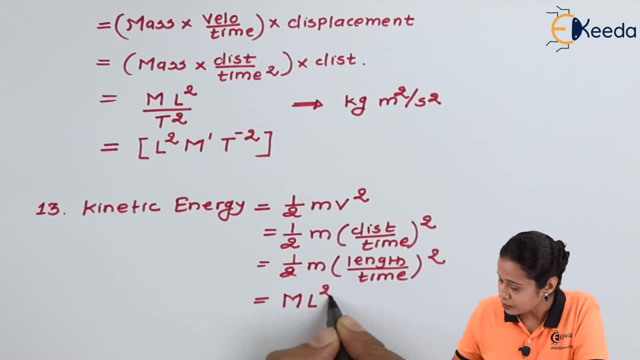 here we will write down m L square upon t square. So if you want to write down the dimensions, we will write down dimensions L square. m1. t is in the denominator, So we will write down t minus 2 square. And if you want to write down the units, units will be. the unit of mass is kg. 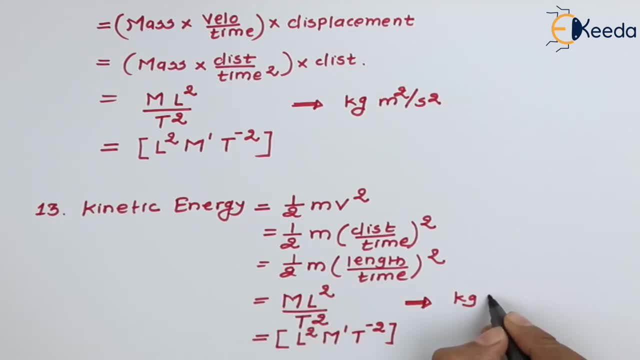 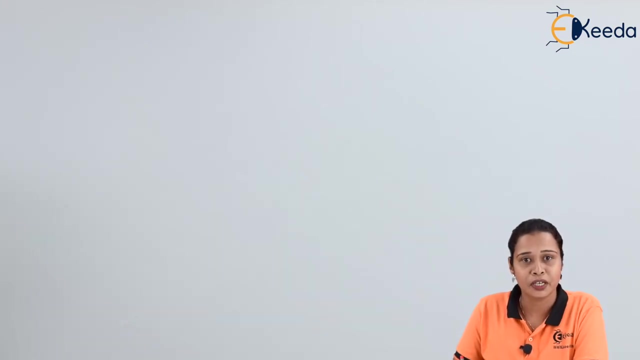 Unit of length is meter. Here we have a length square means meter square upon t square. that is second square. So the unit of kinetic energy is kg meter square per second square and the dimension of kinetic energy is L2 m1 t. Next physical quantity we will take, that is, a potential energy. 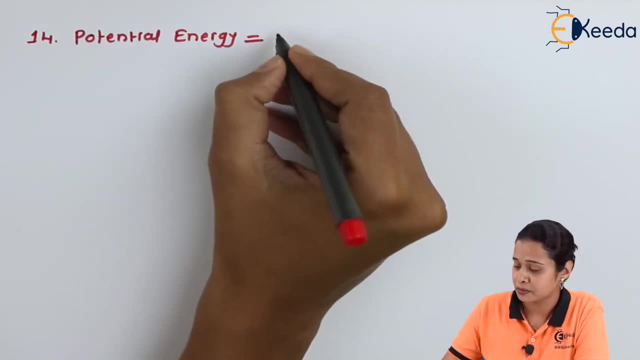 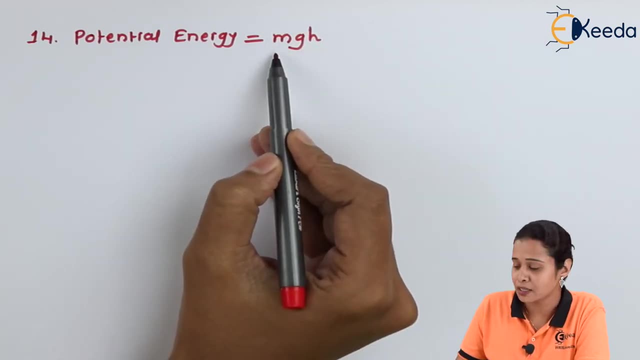 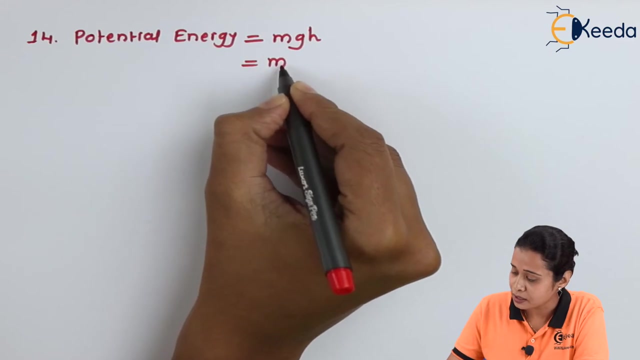 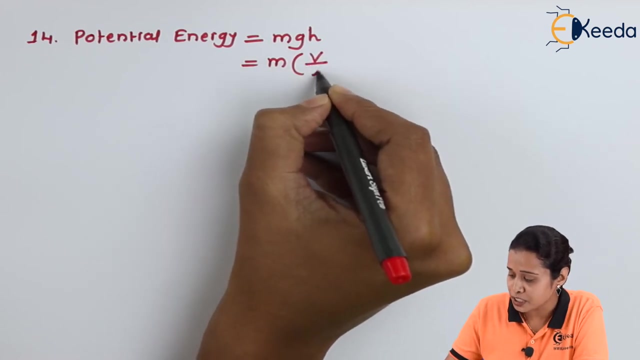 We know potential energy is mgh, that is mass, g and h. H is a height. Here m stand for mass, G is acceleration due to gravity and h is a height. So we will write down here: mass stands for m. Then g is acceleration due to gravity, So we will write down here: velocity per unit time. 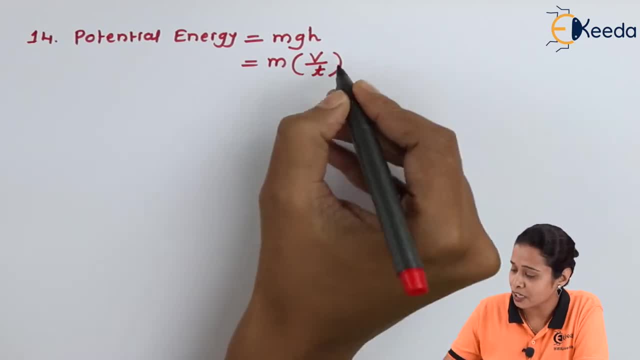 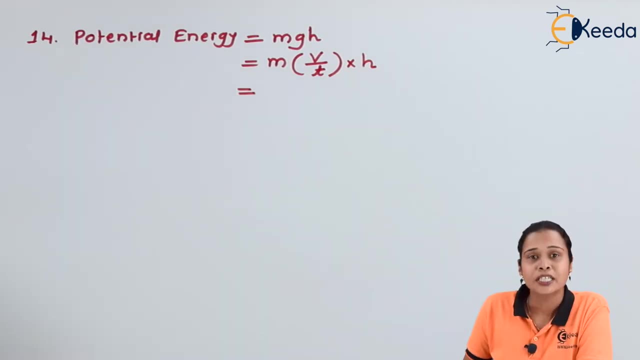 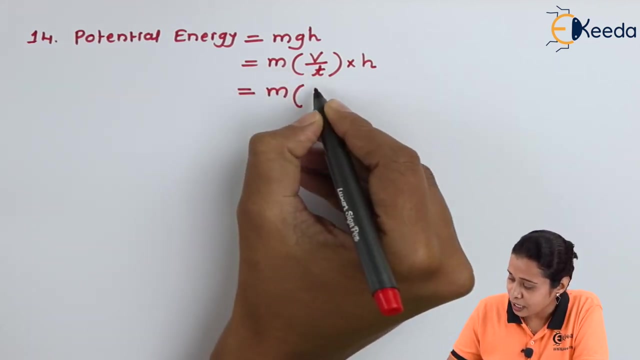 and height is nothing, but it is a length. So we will write down here length or height also, no problem. Now here velocity can be expressed in terms of distance per unit time. So this formula will become m, distance per unit time. velocity means here we will write down distance per unit. 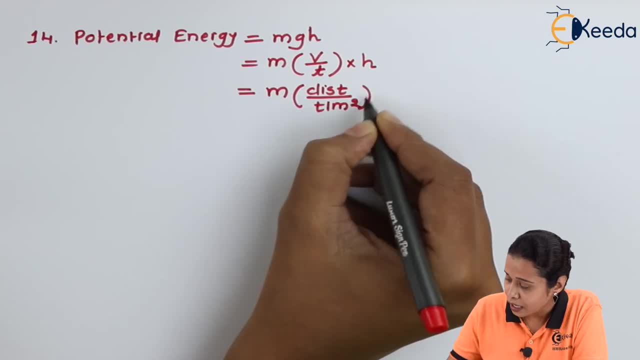 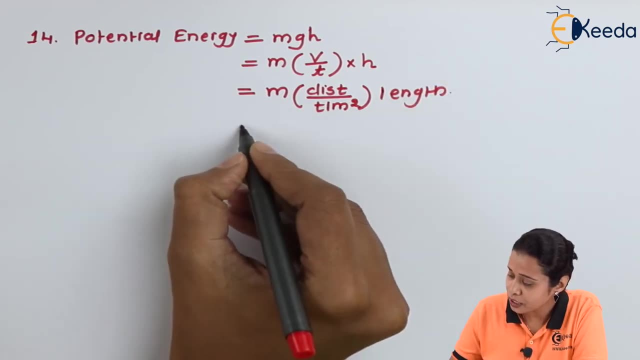 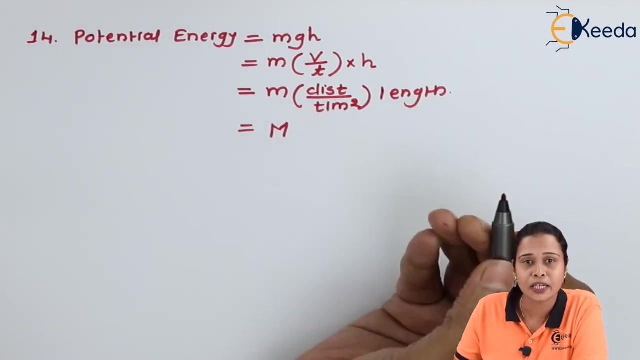 time means again: here we will write down time square. And this height can be expressed in terms of length. So here we will write down m for mass, distance and length. both are the same quantity. So we will write down here L square, and for time we will write down t square. 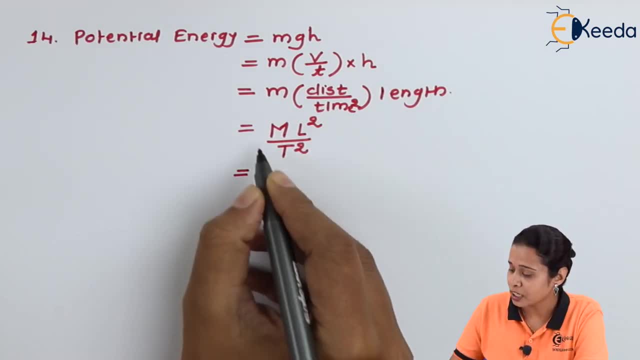 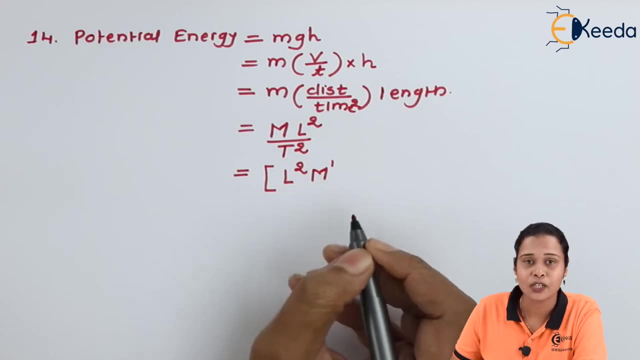 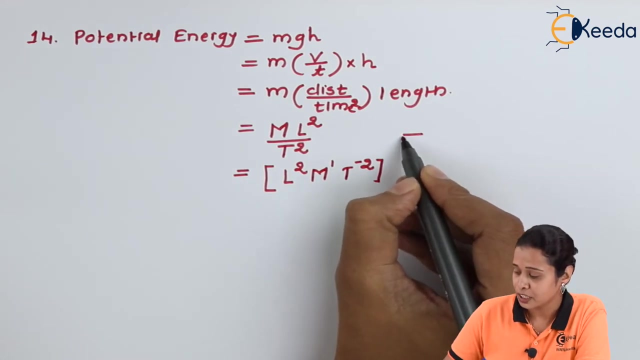 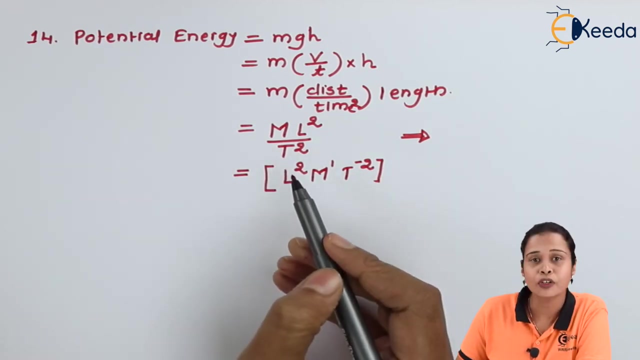 The dimension for potential energy will be L2 m2.. T is in the denominator, So we will write down t minus 2 square. If you want to write down unit for potential energy, we can derive it from this equation. So here m. m is nothing but mass. So unit of mass is kg. 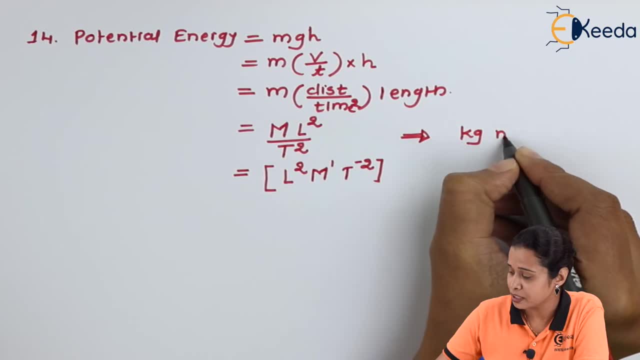 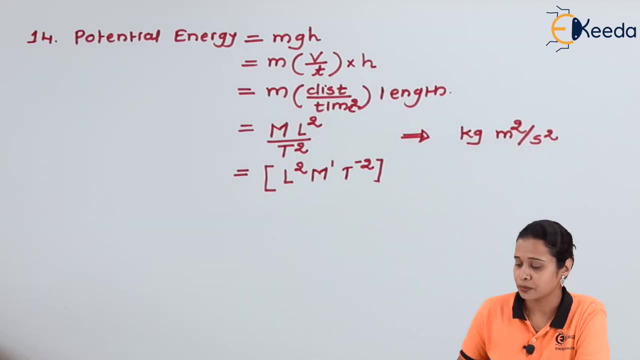 Length. Unit of length is meter, So here we will write down meter square, And unit of time is second, So here we will write down second square. So in this way we can find out the unit and dimension for the potential energy. 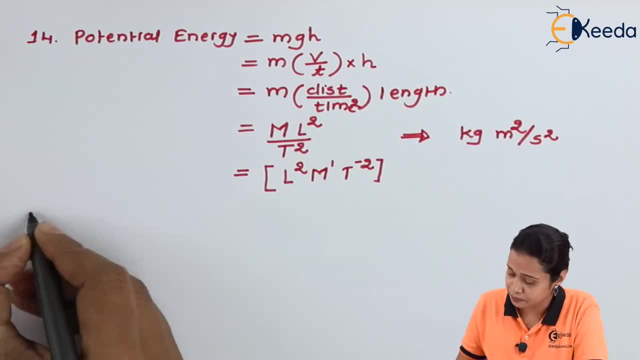 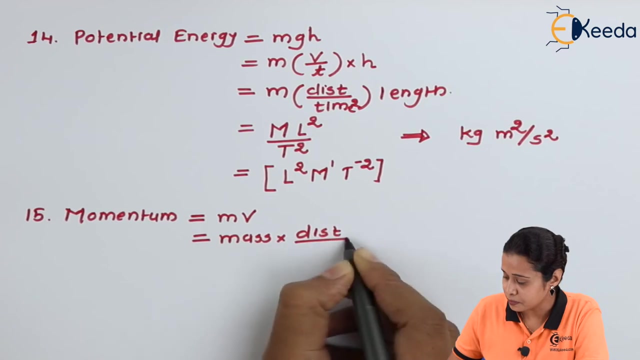 Next physical quantity we will take. that is a momentum. We know momentum is mass into velocity. Now we know velocity is again distance per unit time. So we will write down here mass into distance per unit time. So if you want to express this in the physical quantity, we will write down here m for the 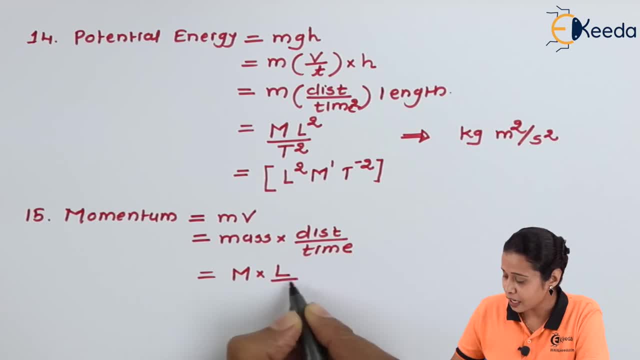 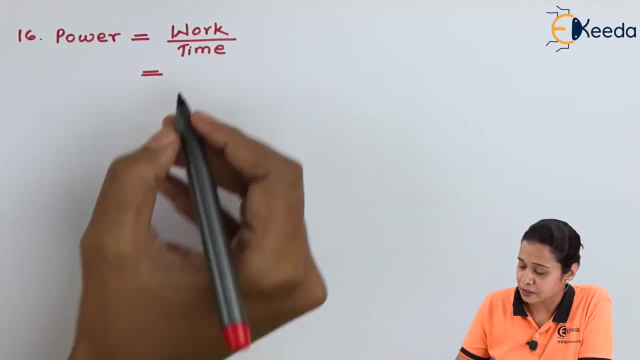 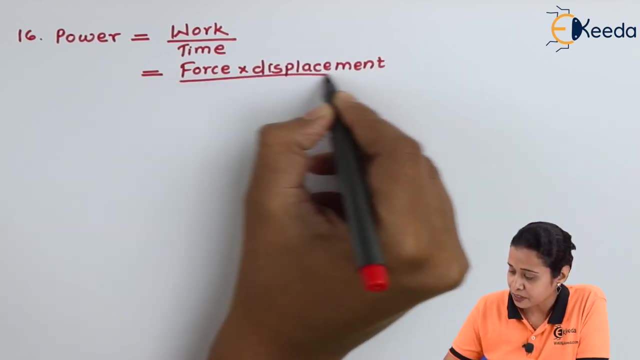 And if you want to write down the units of momentum, you can write down m1.. So this is minus 1.. So this is minus 1.. So now the unity of momentum can be expressed in terms of force into displacement. 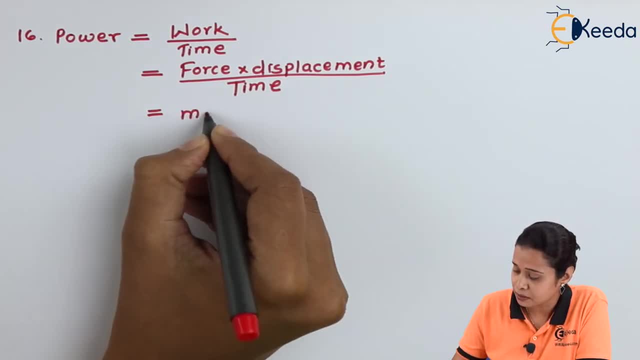 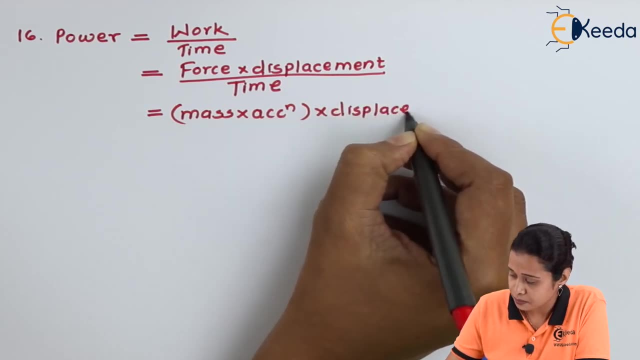 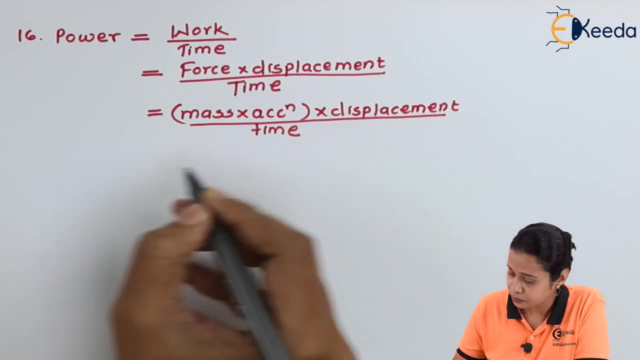 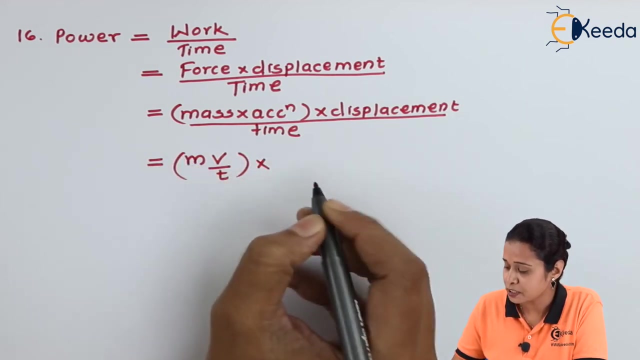 And here we have a time Now force again can be expressed in terms of mass into acceleration, into displacement upon time. now acceleration again can be expressed in terms of velocity per unit time. so here we have a mass into velocity per unit time, into displacement. that is nothing but length. 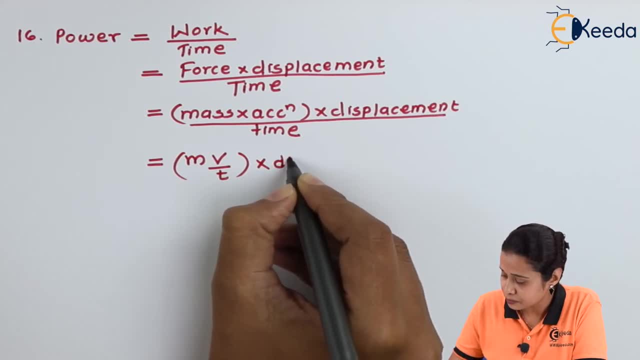 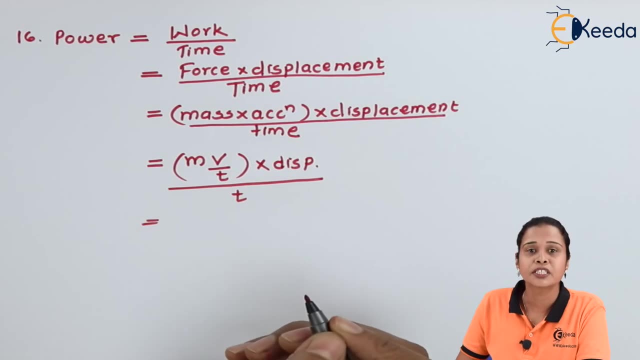 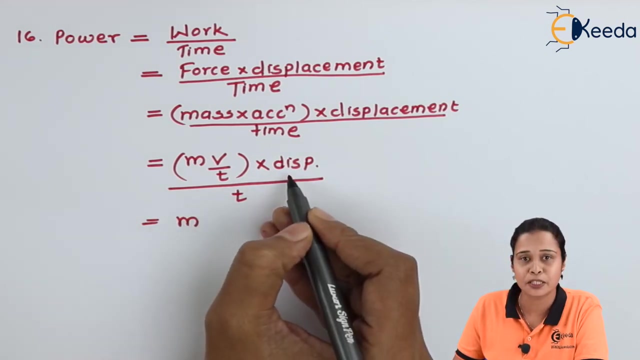 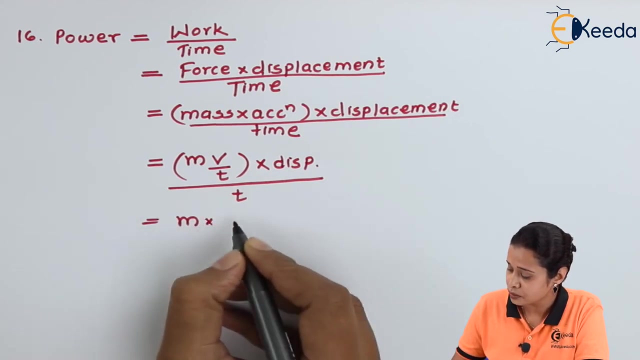 upon time. here velocity is distance per unit time. so directly here we can write down mass into distance. distance and displacement, both can be expressed in terms of length. so here we will write down mass into length square upon t square. so here we will write down mass into length square upon t square. 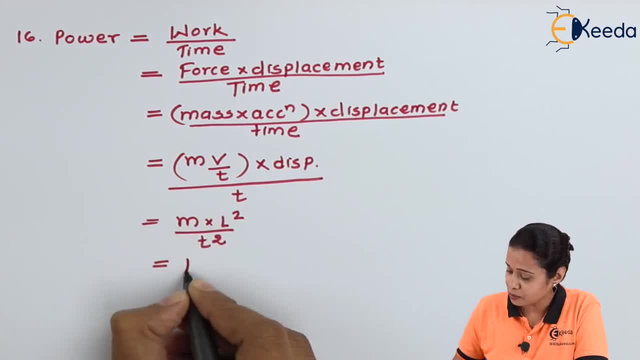 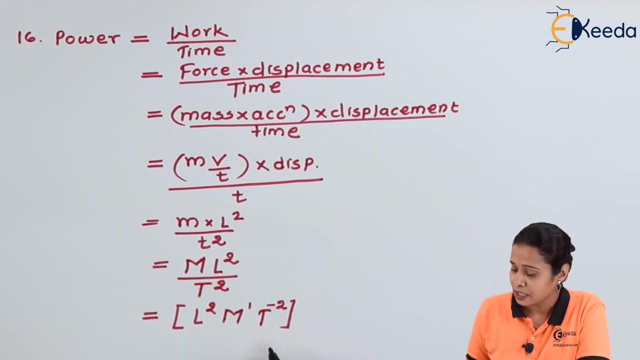 hence we can express this mass in terms of m, l, that is a length, and t, hence the dimension of power, can be written as l2, m1. t is in the denominator, so we will write down t minus 2. this is the dimension of power. suppose we want to find out unit, so we can find. 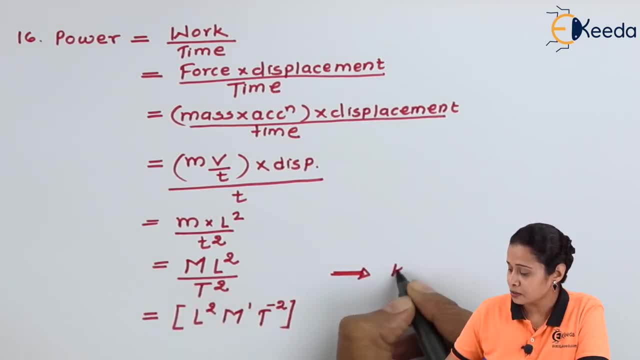 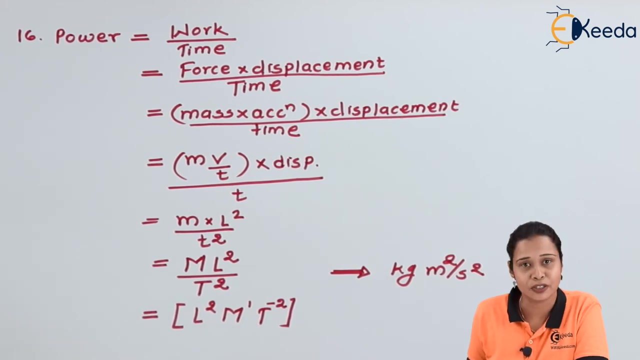 out unit from this formula. so So m is nothing but kg. Mass can be expressed in terms of kilograms, So it is kg. Then we have l. square means meter. square upon t. square means second square. So unit of power is kg meter square per second square, and the dimension of power is l2 m1 t minus 2.. Next, physical quantity. we will 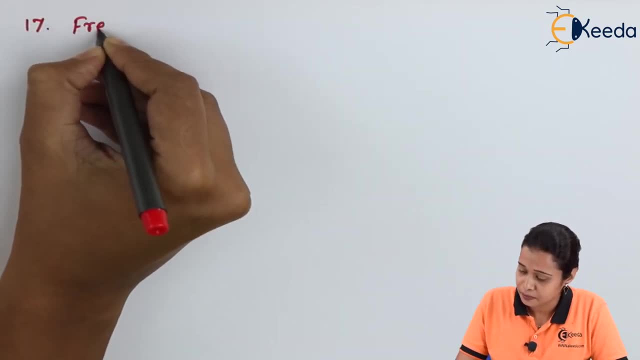 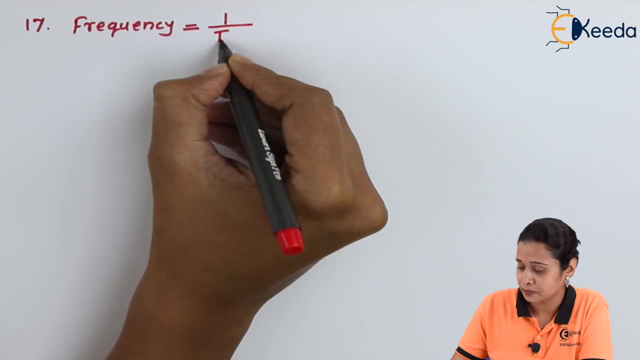 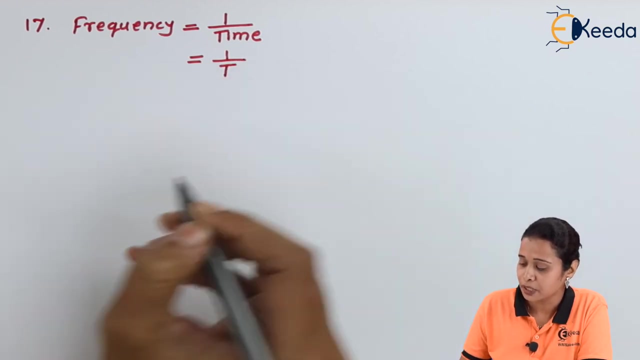 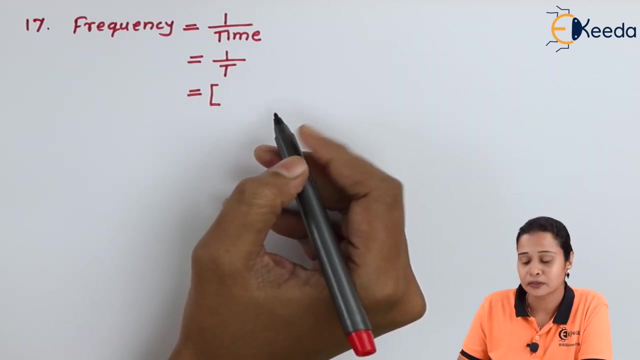 take, that is a frequency. We know frequency is 1 upon time. Time can be expressed in terms of t, So we will write down 1 upon t. Hence the dimension of frequency is here length and mass. both the terms are absent. So here we will write down l0, m0.. 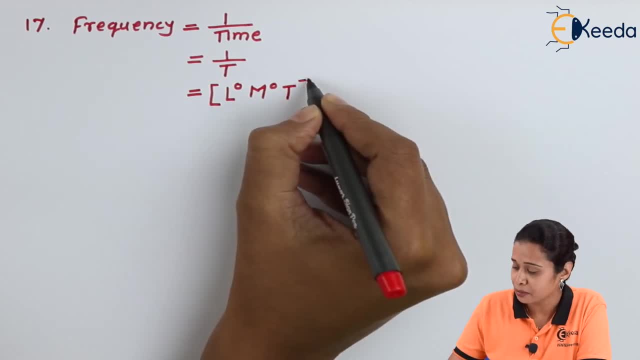 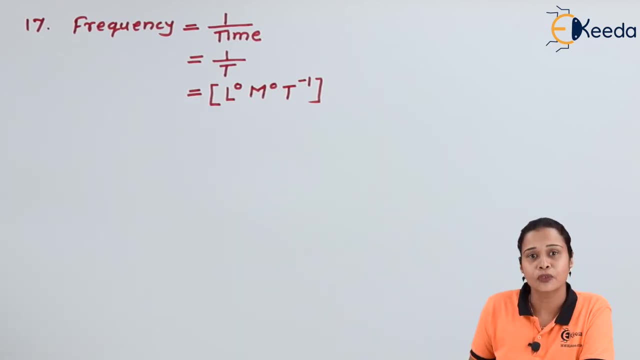 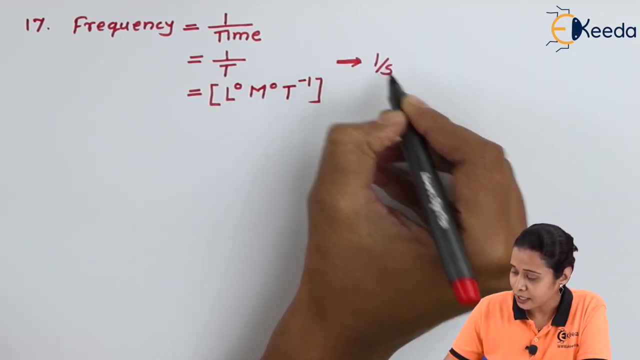 t is in the denominator, So here we will write t minus 1.. This is the dimension of frequency. If you want to find out the unit of frequency, we can find out from this formula. From this formula we can write down 1 by second. or here we can write down second inverse per second. It is a. 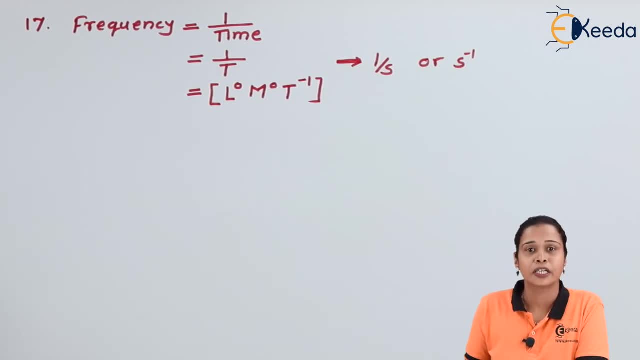 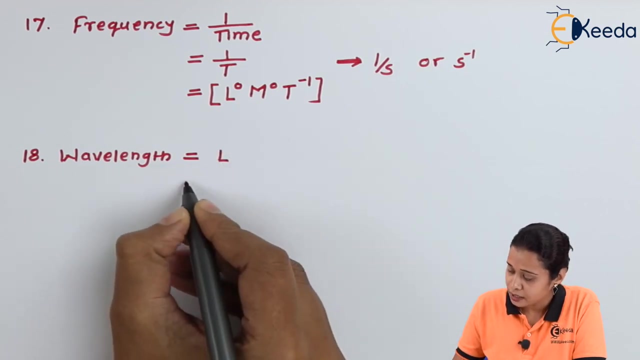 unit of frequency. Next physical quantity we will take, that is a wavelength. We know wavelength is nothing, but it is a length of one wave. So length we will express in terms of l. So here only one quantity is present, that is a l. Hence the dimension of this physical 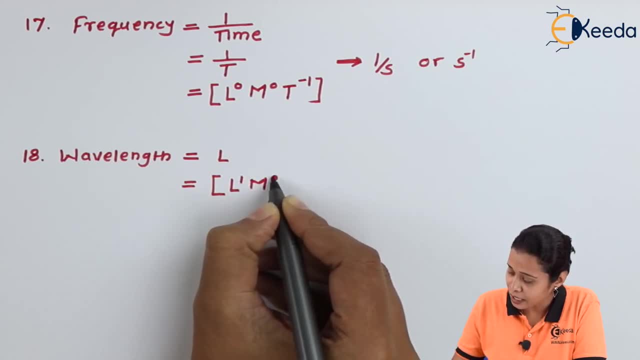 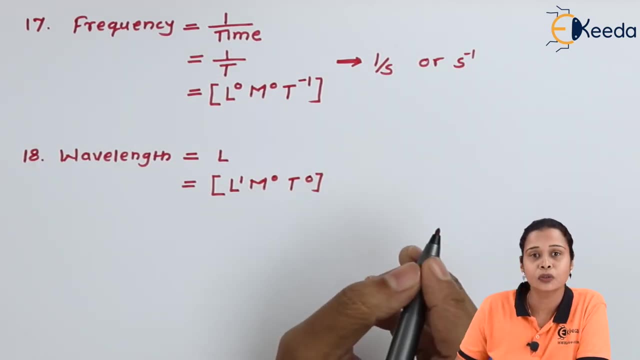 quantity: wavelength is l1.. Mass and time, both are absent, So m0 or m0 t0.. And if you want to write the unit of wavelength, we can write down from this: that is a meter. Next, physical quantity we will take, that is a trace. Trace is nothing but force per unit area. We can express force in terms of. 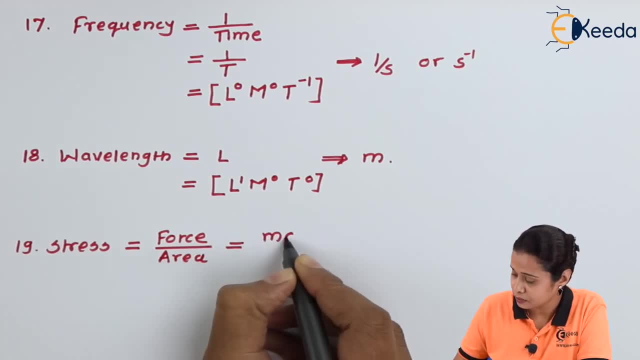 mass into acceleration Area in terms of a, That is capital A for the area. So here we will write down area. Then again we have a acceleration. Acceleration can be expressed in terms of velocity per unit time, So here we will write down m, velocity per unit time upon area. 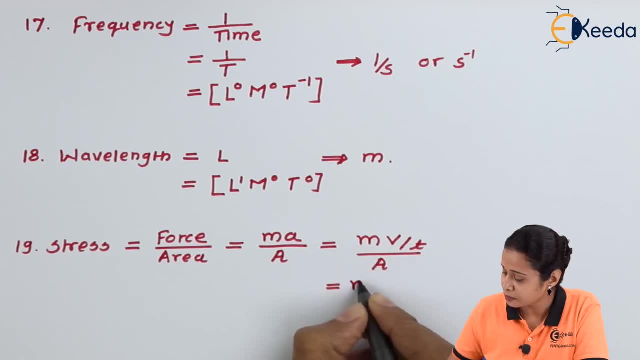 Now, here we will write down: mass Velocity can be expressed in terms of distance per unit time. So here we will write down distance Per unit time. Time is also there, So t square upon area A. So if you want to express these terms, 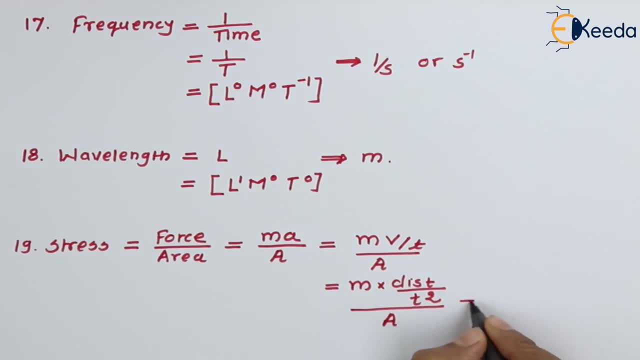 in terms of the fundamental quantity, we will write down here: m. This is for the mass. Distance means l upon t square area. Area is nothing but length into breadth. So we will write down here l square. Here l will get cancelled. So finally, here we have. So dimensions are here. We can consider l. 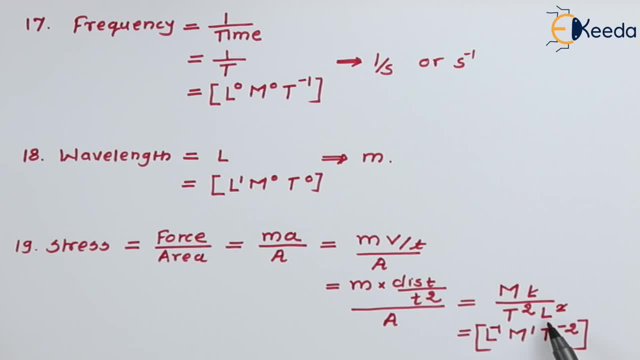 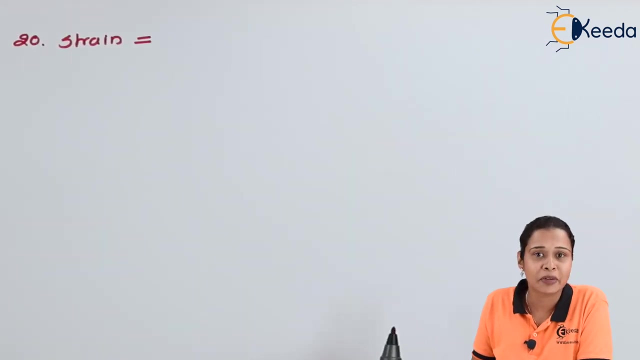 minus 1, because here in previous equation l is in the denominator. So here l minus 1, m 1 and t minus 2.. These are the dimensions of trace. Next physical quantity we will take. that is a strain. We know strain is change in dimension upon original dimension.